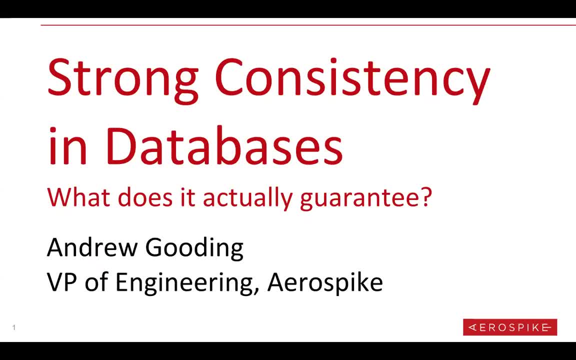 consistency. We tried a very novel approach to strong consistency which seems to have worked out really well And we'll get into some of the a little bit about what's novel about it. But the talk really is not primarily about Aerospike's strong consistency, It's really about the 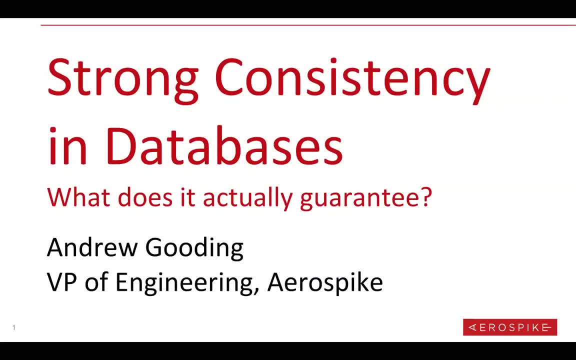 consistency. It's just a talk about strong consistency in general, what the trade-offs are with high availability, what it really means, what your concerns might be, choosing between the two and, just in general, what it guarantees. So I gave this talk last year in Israel and I was literally 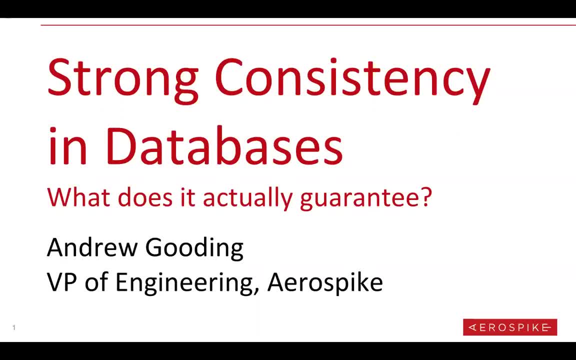 not allowed to mention Aerospike During the talk, So you'll see, it really is a very general talk, Although at some points I do. I will mention Aerospike's implementation, just to highlight the fact that you don't necessarily have to do things one way or the same way to achieve strong consistency. So, again, the talk's really just about. 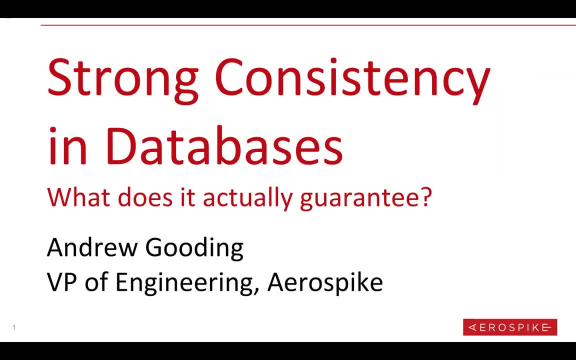 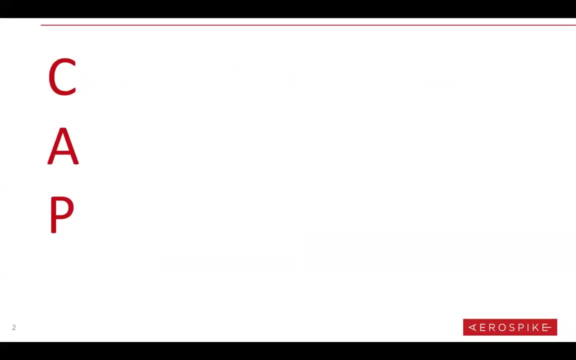 strong consistency in general and the trade-offs compared to the alternatives. Okay, A good place to start is the CAP theorem, which, if you have not heard of this, it is a theorem that states there are three things in a distributed system database: strong consistency, which the 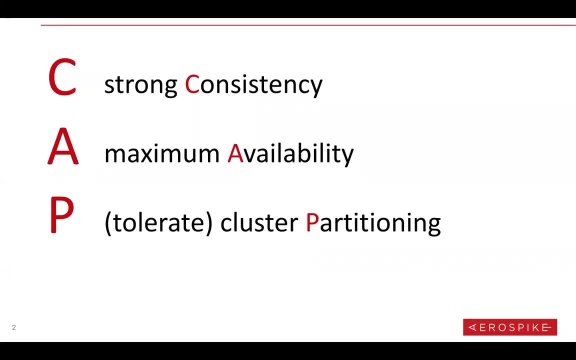 subject of this talk mostly maximum availability, which we'll also talk about a bit, and toleration of cluster partitioning And the theorem which I'm not going to prove here, but as the talk goes on you'll kind of get the idea why this theorem is true. The theorem says that you can only get two of 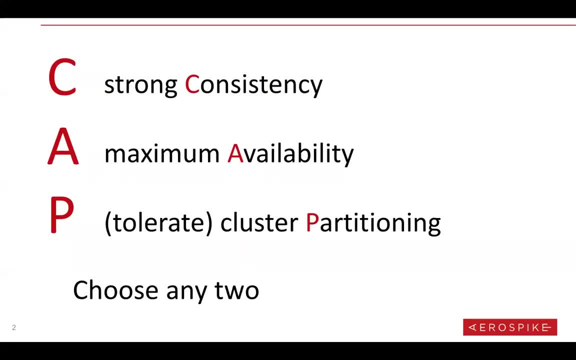 these three. You can't have all three. And again, as the talk goes on, it will sort of emerge why that's true, So I'm not going to bother prove it here. You can look that up If you really want to see it. So yeah, you can only choose two of these, And of course, in the real 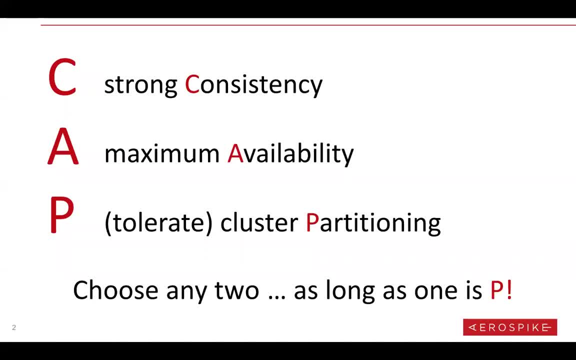 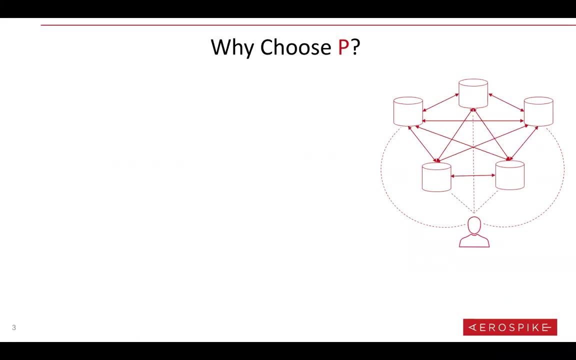 world. one of the two you're going to be choosing is P, meaning that this really is going to boil down to a choice between which you're choosing- between C and A. So why do we choose P? Or why do we have to choose P? And the reality is we're going to have to choose P, And the reality is we're. 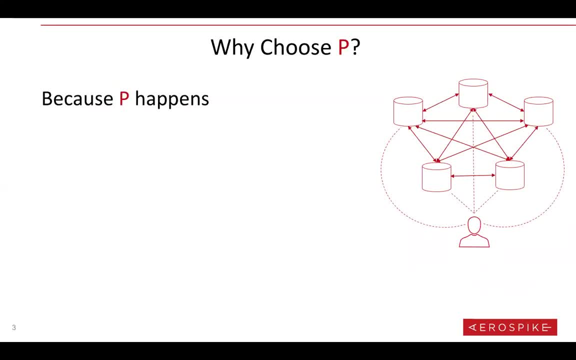 going to have to choose P, And the reality is that cluster partitions in real distributed systems do happen. You're going to see nodes crash And you're going to see connections in your network break, And the reality is that, even if you have a really, really good system, someday, somehow this is 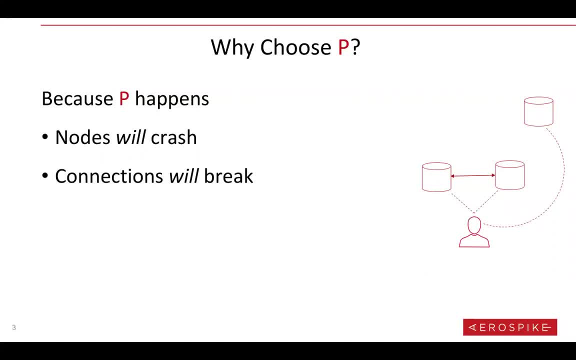 going to happen And you're going to end up. it's going to. it may be important. we're going to have to look at whether you decided to choose C or A in this scenario. So let's see Some other terminology. I. 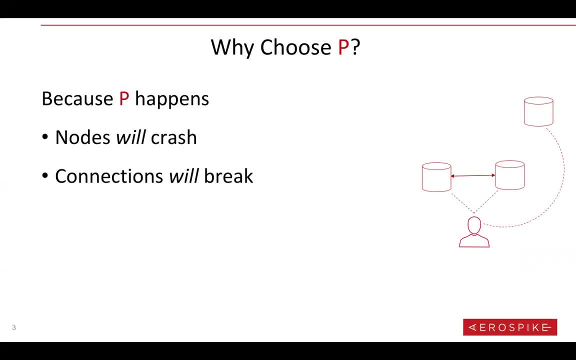 might introduce, in case I start spewing slang through this talk. When connections break, you might often hear me talk about a split or a split brain. That's a scenario where the user application, via a client, can only see one node. Everybody can see pieces of the cluster, but they can't see each other. 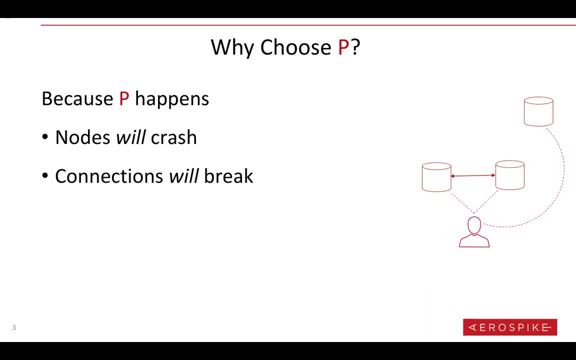 Sometimes also the clients won't be able to see certain pieces of the cluster. But that's what we mean when we say cluster splits or split brains. When nodes split off, if they're completely disconnected by a network, it's more or less the same as if they did go down. They're no good to anybody if the application can't see them completely, And it makes sense to say that if someone 잘 Divinekiem auf der Erde 아니에요, wird functionen. If the application fails, and fails in an area it's going to be useful, A set of tools are tools. 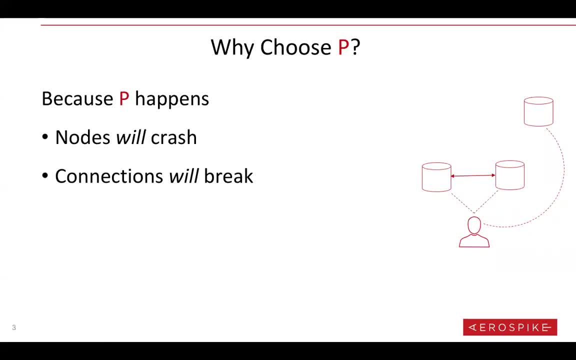 But we don't know what. And the reality is we can measure potential, similar thoughtfulness, And it certainly we do have to. and if other nodes can't see them, But sometimes nodes just literally will go down too much as we'd like to think, we can write perfect software. 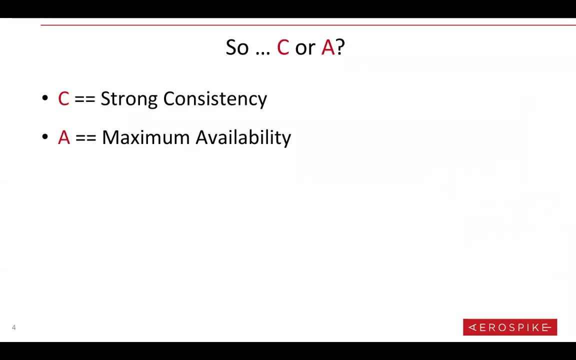 Some other things to clarify about our choice between strong consistency and maximum availability. Strong consistency does have a very clear definition which I will explain shortly. And maximum availability? I've heard different definitions of it. My definition is pretty much: if you can see any part of the cluster, any node, 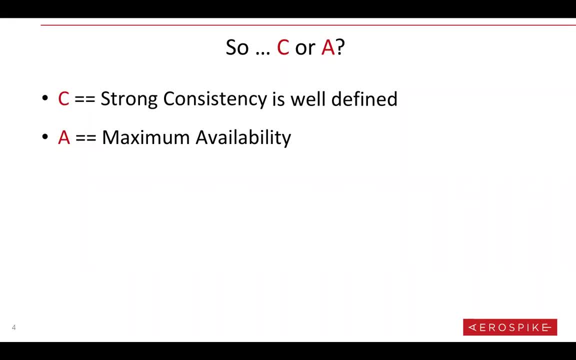 then transactions are allowed to proceed. Now note that maximum availability doesn't mean 100% availability. If you can see a node, even if you decide I'm going to choose A and I'm going to have a highly available system if all your nodes go down, 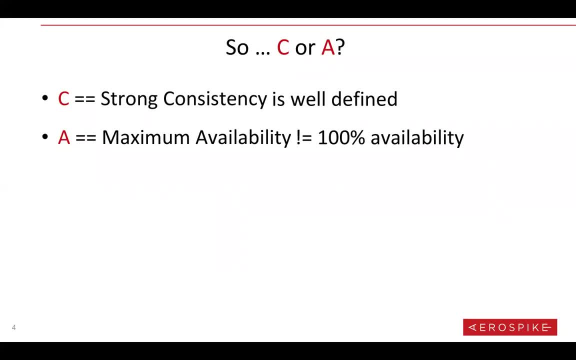 I can tell you that your availability will actually go to zero, even though you've chosen A. So maximum availability just means that pretty much you're going to take any availability that you can get, meaning if any node is visible, we'll let transactions through. 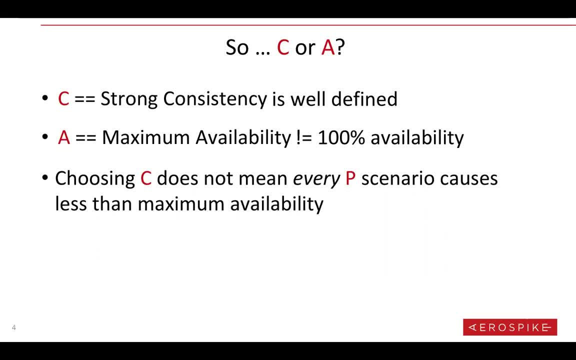 Also, I want to point out that just because you're making this choice, it doesn't mean that every situation in which you have a cluster partition will cause you to give up the other thing that you're choosing not to have. So choosing strong consistency does not mean. 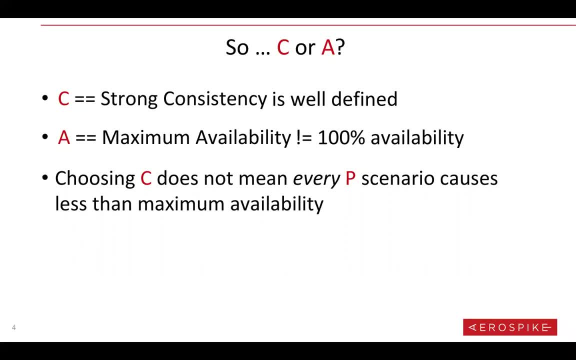 that every situation causes you to decrease, to be less than maximum availability, And likewise choosing a highly available system. choosing a highly available system, choosing a highly available system, doesn't mean that every partition scenario necessarily breaks strong consistency. So a good distributed system, for example. 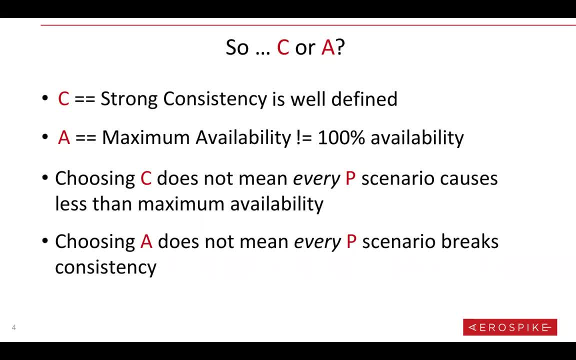 should at least allow you to upgrade where you don't lose either C or A, meaning you should at least be able to take a node or perhaps more nodes down in sequence to upgrade your software without any loss of availability or consistency, And that that 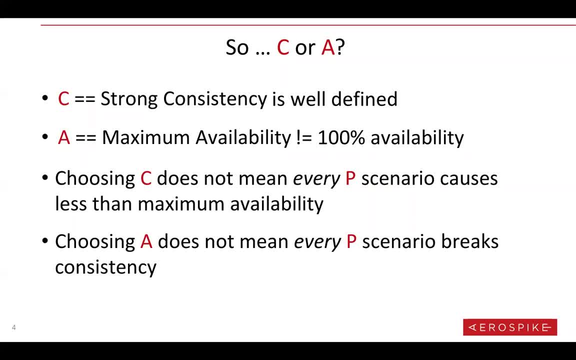 that's for us. when we were developing our SC mode, that was pretty much the primary criteria- is that we have to make it so that our availability loss is zero during normal, what we call normal upgrade- scenarios. So yeah, it's not always that the first thing that happens. 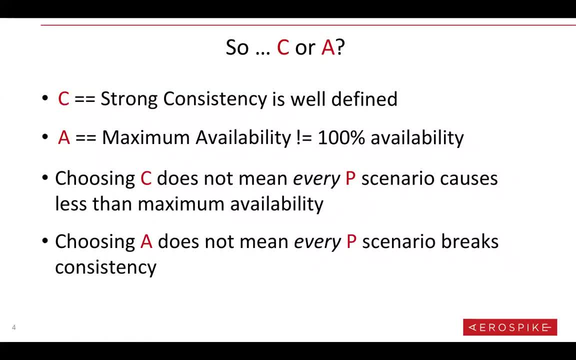 you know, any node going down means that you're going to lose one or the other of A or C, depending on which one you choose. Okay, so I said I was going to define strong consistency. So my definition, which I think is pretty well agreed on in general, 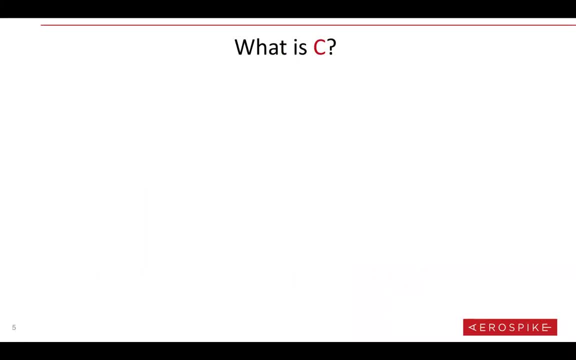 is that what you must see in the cluster is a single linear progression of a record version. By the way, for this whole talk, I'm really talking about single record transactions. If you have any questions, please feel free to reach out to me. 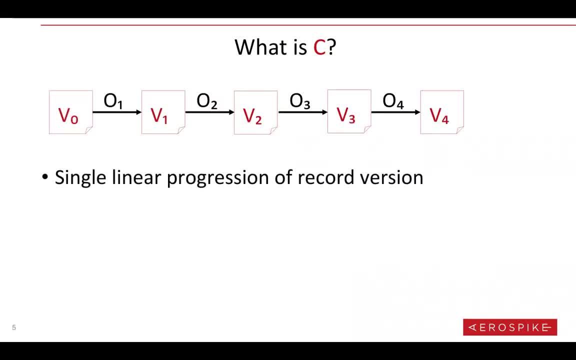 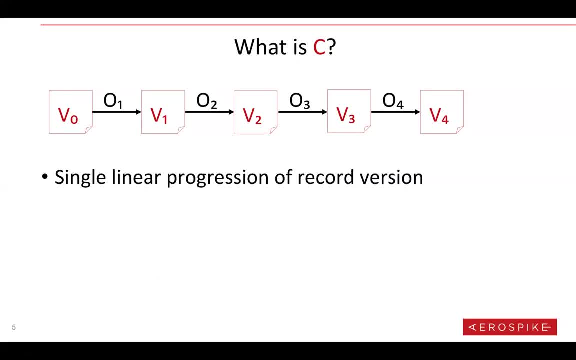 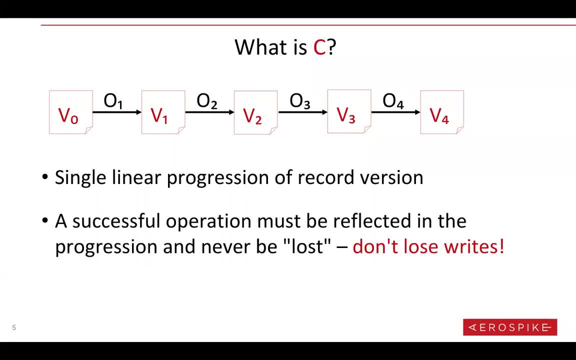 so so. so Corollary is that any successful operation has to be reflected in the progression and never be lost. So once you've done something to affect a record and the database told you that that operation succeeded, you can't ever after that encounter a version of the record where it was as if that operation didn't happen. 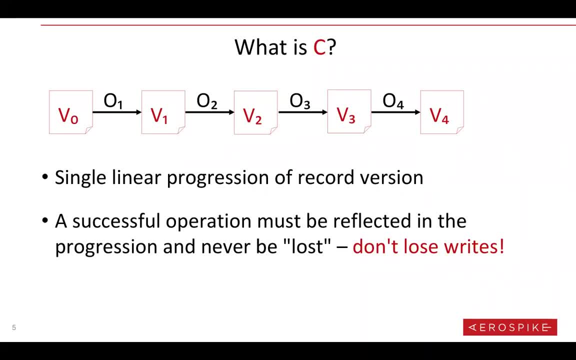 So to me, this is really the primary definition of strong consistency. We guarantee that you will never lose a write. Notice also that our operations here they don't necessarily have to be literally an atomic transaction, an operation in an atomic transaction. It could be a read-modify-write, which is two transactions where the write is optimistically reporting the generation that it read. 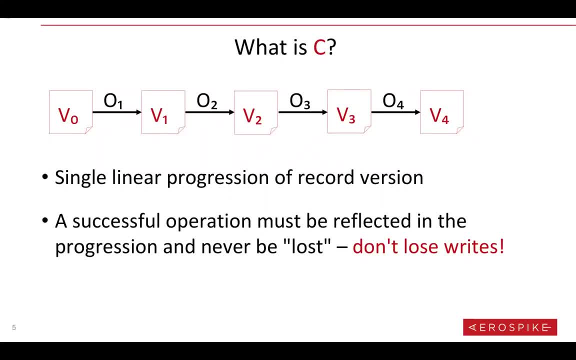 and will fail if it's not encountering the generation that it read. So it works. The operations can be a read-write combination or they can be an atomic thing, where it's just one transaction that takes the existing version of the record and, based on that, generates the next version of the record. 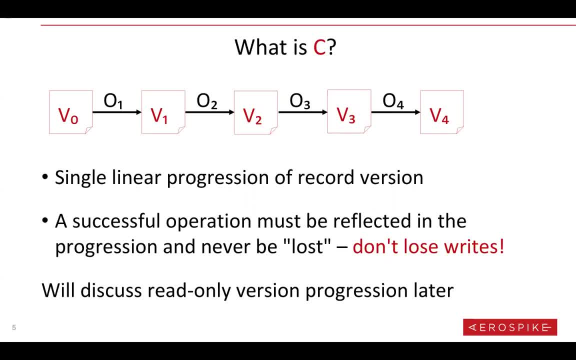 Now my definition is all about writes, which of course involves looking or reading the previous version of the record. I'll defer talk about read-only version progression. We'll talk about this definition a little bit again then, but for now I want to keep clear that when I'm talking about strong consistency, 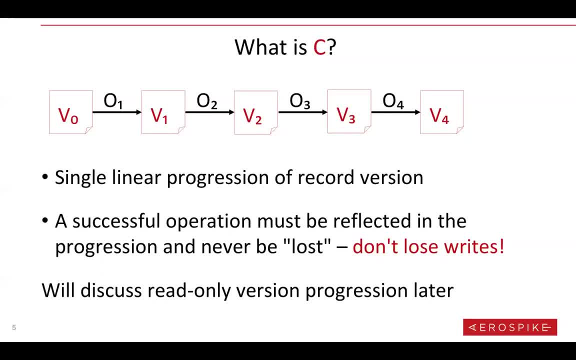 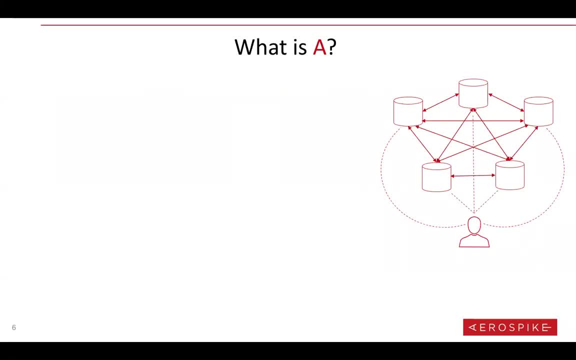 essentially my view of it is: I'm not losing writes. Okay. so what's high availability then? High availability means that operations, as I said earlier, will succeed as long as any part of the cluster is visible. So I'll take the operation and I'll do it. 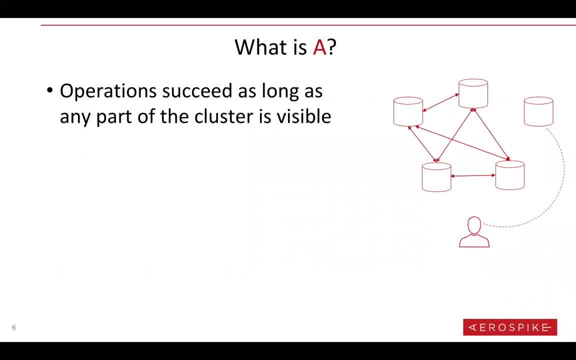 It doesn't matter. even if the situation is that I can only see one node and it can't see any of the other nodes, I might still decide that, yep, I'm going to let you go ahead and do a transaction. What it means is that you can have- you're going to violate that linear progression that we defined, that single linear progression that we defined. 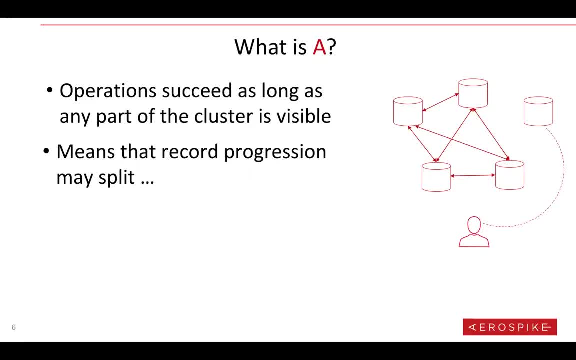 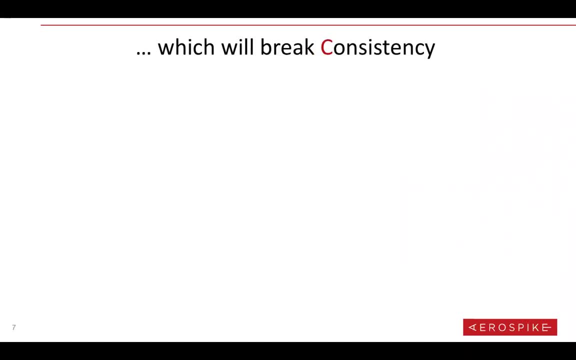 It was the basis of strong consistency. So the record progression can now split, which will break strong consistency. So to redraw our original sequence where we had operations 01 through 04, starting at version zero, if operations 01 and 04 happen in one split of the cluster and operations 02 and 03,. 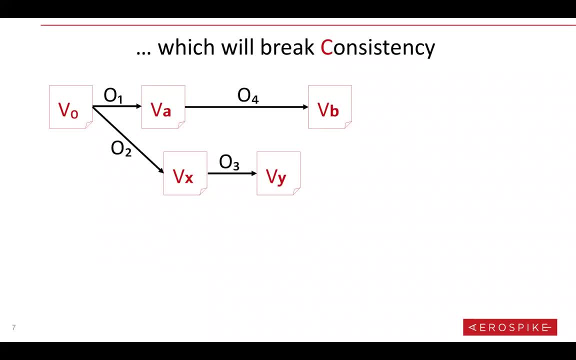 happen in another split of the cluster, then you end up with these versions, which are absolutely not. none of them will be the same. Well, maybe VA will be the same as the one, the first one that you saw in the strongly consistent sequence. 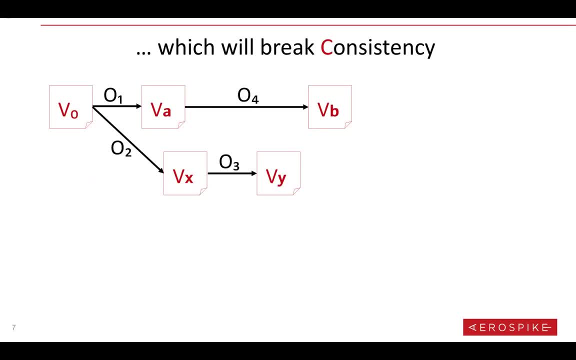 But in general, here you're going to end up with scenarios where you have different versions of the record in the cluster which you can see in the versions are not the same as what you would have if they were strong- strong consistency. In other words, you'll be missing rights. 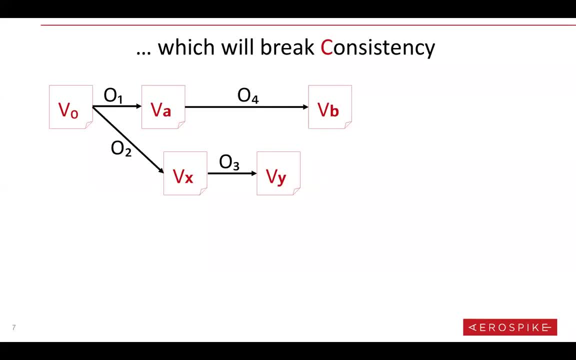 VY will be missing rights 01 and 04, and VB will be missing rights 02 and 03.. And this is irrevocably breaking strong consistency. It does not matter if somehow we magically are able to recover V4, as it would have been if this whole situation never happened. 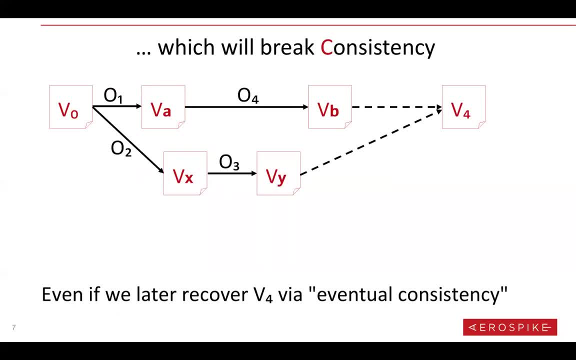 So some people will call the scenario where we actually do recover V4 eventual consistency- And I'm going to put my rainbow powered unicorn up here, not because I don't believe that eventual consistency is a real thing, but there is a lot of mythology surrounding it. 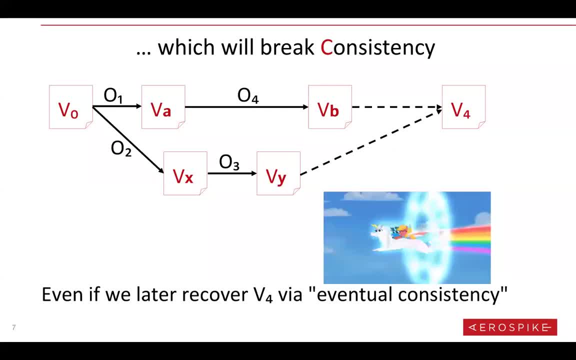 And we're actually. it's probably good for us to spend a few slides talking about what this really is. So the first big myth that I see around it is this conception that it's somehow a step along the way to strong consistency. So I've had discussions with customers that sound like the following: 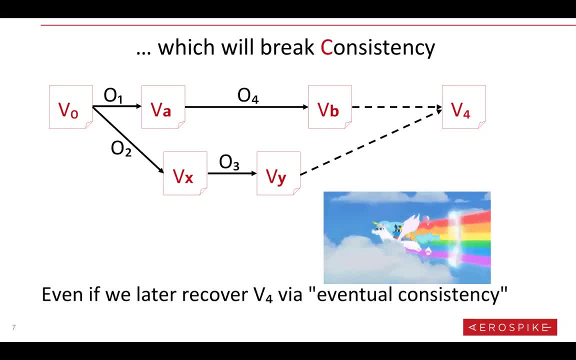 The customer will say: well, for this particular use case we'd like strong consistency, but we can make do with eventual consistency. So it's okay, if you can't deliver, deliver strong consistency, we'll settle for eventual consistency. And 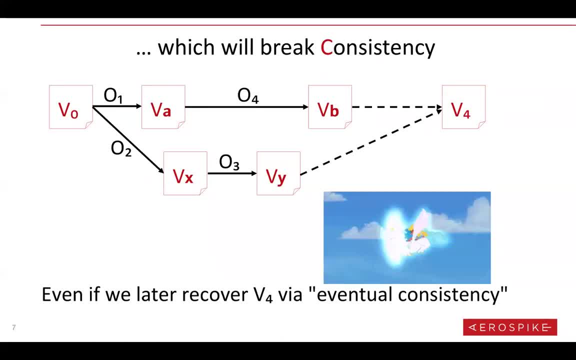 you know I'll ask them wait. do you prefer eventual consistency, Meaning the increased availability in these scenarios, or do you prefer a strong consistency? And they repeat: well, I prefer a strong consistency, but we can. we can manage without it. 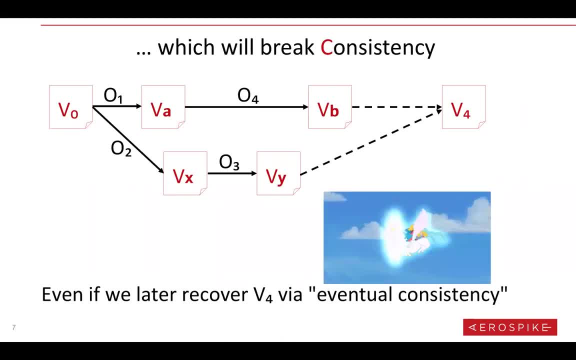 It's okay if you just give us eventual consistency And the myth there is the word just It's a it's in their mind. maybe it's a stepping stone on the way to strong consistency, but in terms of implementation and what it entails, 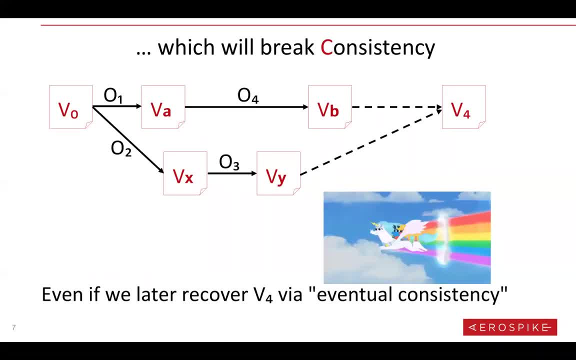 it is absolutely not a stepping stone to strong consistency. They are very different things in principle and they take very different techniques of implementation to accomplish, And eventual consistency is actually every bit as as difficult, in arguably more difficult to do than strong consistency. 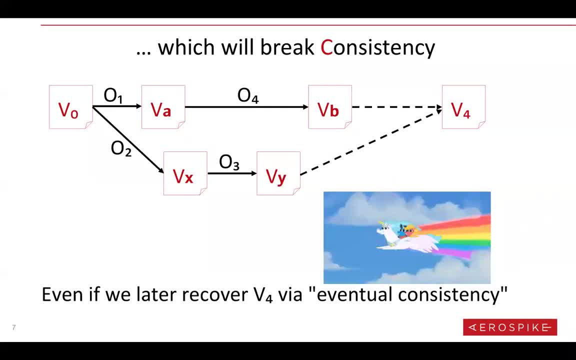 The other thing about eventual consistency is it's often slung around as a general term, as if I really can always easily just recover V4 without any data loss or without you know again, as if nothing in between happened. But in reality 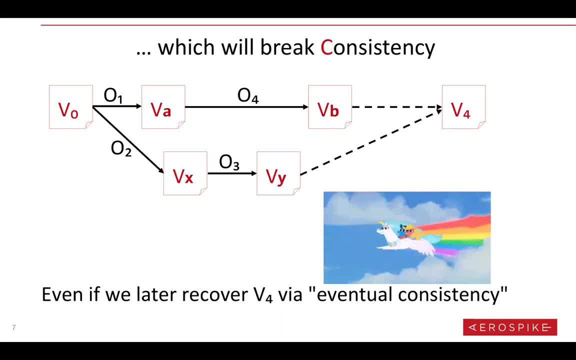 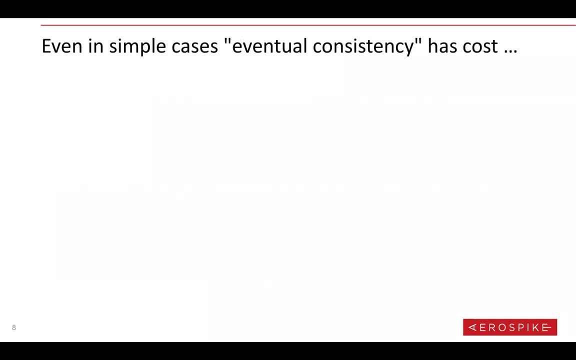 most models of most practical implementations of eventual consistency are incredibly use use case specific. It turns out to be really hard to do it generally. So let's talk about why. Even in very simple cases, you'll see that to do eventual consistency is going to have some extra cost. 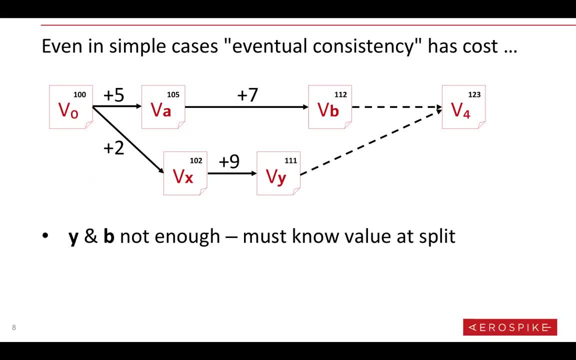 For example, I'm showing a situation here where our operations are just arithmetic addition. So you're just incrementing some number, the, the value of the. the record is just a number And you can see here that just knowing the end states of two splits. 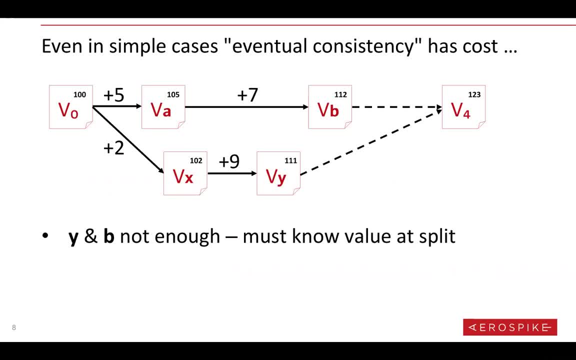 like VB and VY, is not really enough information to recover what, what the record should have been if none of this happened, the V4. You can't tell from those values- 111 and 112, that when you merge them together. 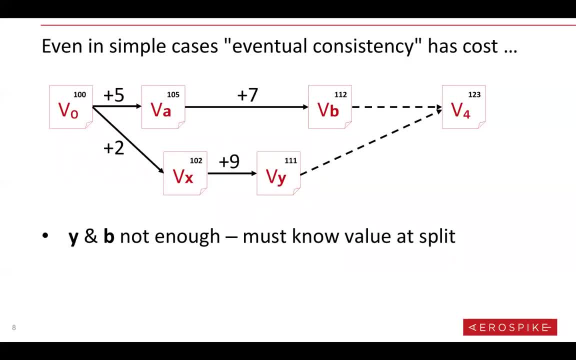 the value is supposed to be 123.. So you have to know. you, in this scenario, at least have to know what the value was when the split happened, And remember that you know this is a simple splits. There could be many splits. 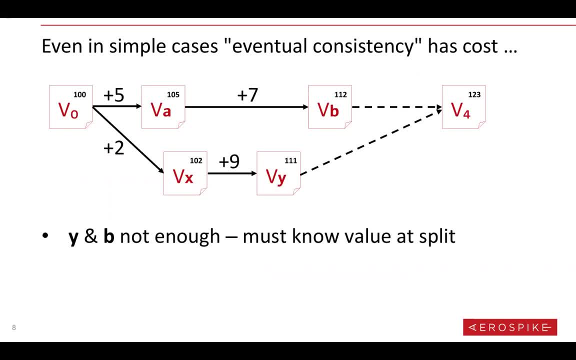 cross merges between splits before you have a final merge. You can have splits where there is no version of the record to begin with that You have to merge back. so it can get pretty involved And in general, to do even this case you have to know what the versions and values are at the splits. 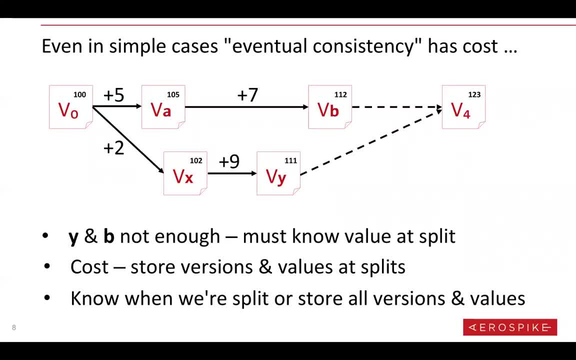 Alternatively, of course, you also have to know when you're split, or you literally have to store all the versions and values, And even things like knowing when you split, in other words, when you can trim your history to start from scratch- is. 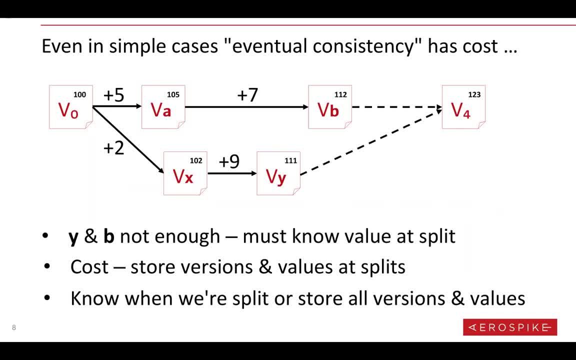 is a pretty involved thing. So even a simple case like this, you're going to end up dealing with history. Essentially, you're going to end up dealing with state and history to be able to recover the version of the record that you want. 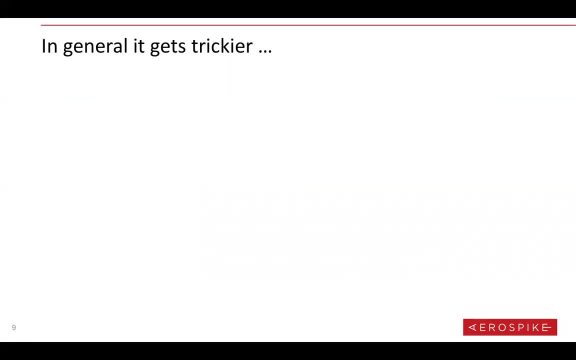 And if you are really trying to do things in general, it gets even worse because in general you can't operate, you can't derive operations from values. even if you know what the original value was and what the final value was, you don't really know what operation got you there. 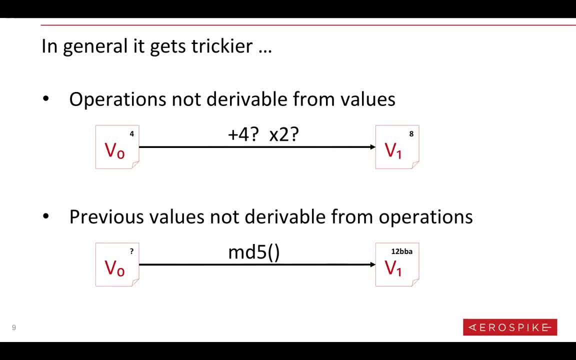 And conversely, just because you know what the operation was and the final value, you can't actually derive the the original value And notice. in this case I put a hash there as an example, but you know many things do this like mods. 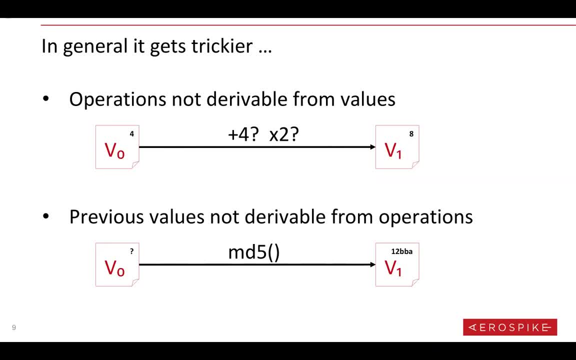 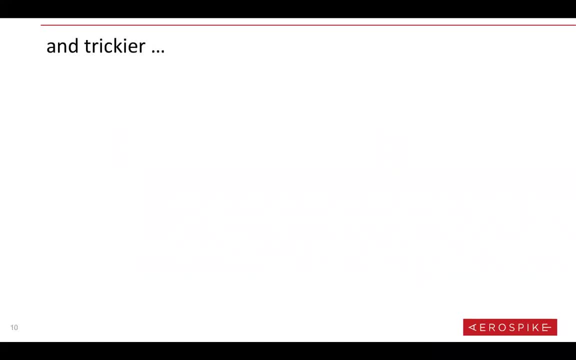 just trimming, selecting it. You can do there any number of things that essentially lose you information irrevocably. So it can be even worse when operations don't commute, because even if you know the operations and you know the values, it depends what order they were applied in. 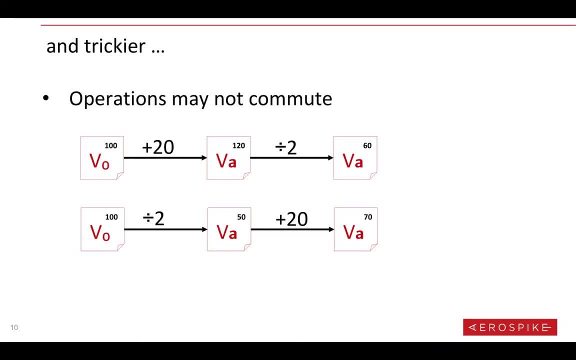 And again here I've done this with arithmetic to show you that two things that don't, that aren't switchable, but it's a lot more common than you think. Even simple things like concatenation: If I start with a string cat and I append woman and then rules. 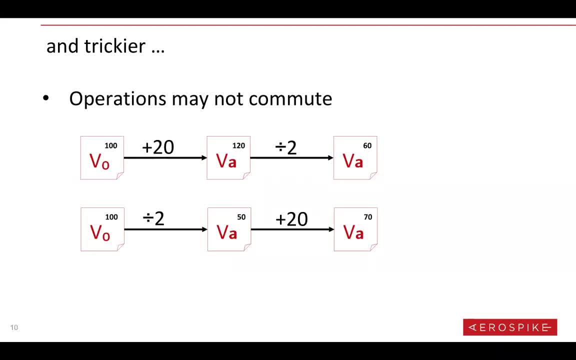 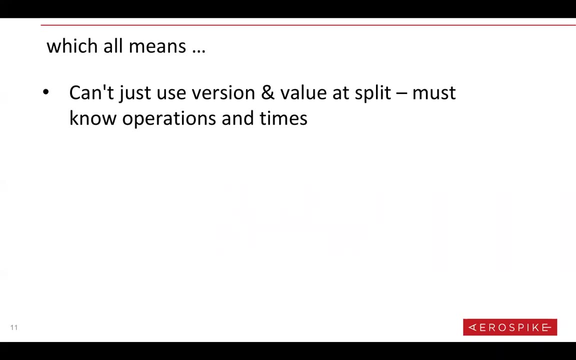 it's very different. you know whether you get cat woman rules and cat rules woman. So you're going to. you're going to see this problem in a lot of use cases. So what all of that means is that it isn't even enough to know the versions and values at the split. 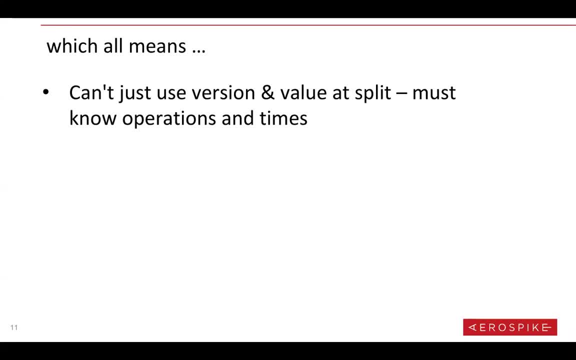 You have to know every. in general, you would have to know all the operations and the order in which they were applied in between and all the splits. So that's a lot of cost to store all of that, to keep all that state and information and history, to be able to accurately recover the version that would have been, if none. if the splits never happened at all, And maybe for some databases that actually might not be a big ordeal if they are already storing multiple versions of records and histories and accurate transaction IDs or operations logs. If they're already doing that for other reasons, then maybe this is actually not that. 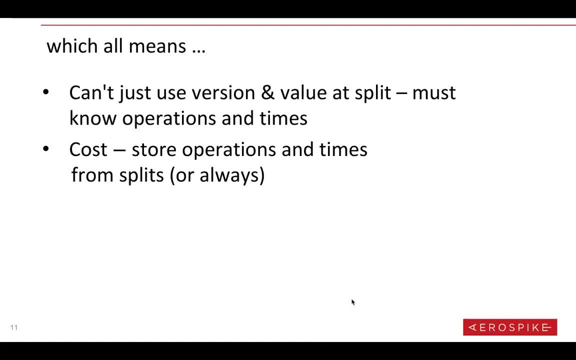 that much of an extra chore, But for some databases like like ours at Aerospike, we only store one version of the record, the latest version, And we don't don't have an operation log, And so for us this would actually be very 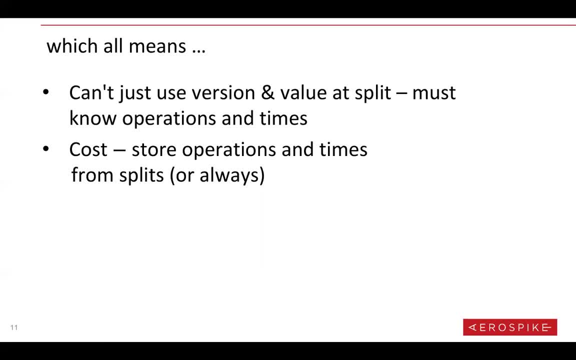 very difficult to do. It would be very costly and very different. You'll often hear the words CRDTs slung around, like well, why don't you just use CRDTs or use emerges? But those are really just names that package everything I just said. 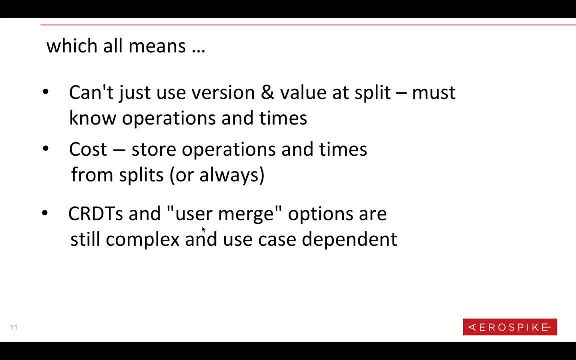 A CRDT will be a way of storing the necessary history and information to do resolution for a particular use case. CRDTs in general are are also well again, because they're eventual consistency, they necessarily are. notice that they're not. 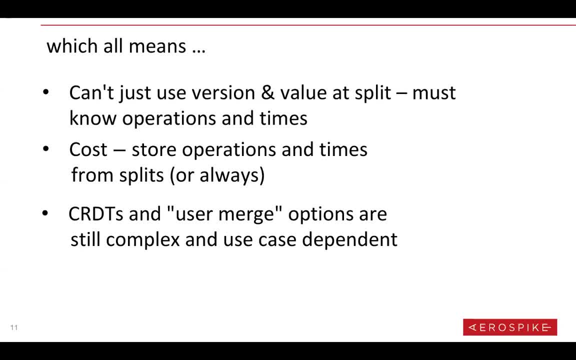 don't let anyone kid you- They're not giving you strong consistency. And also- don't let anyone kid you- They are always very use case dependent. So when you're going to use a CRDT, it'll definitely be a CRDT that caters to a certain kind of operation or 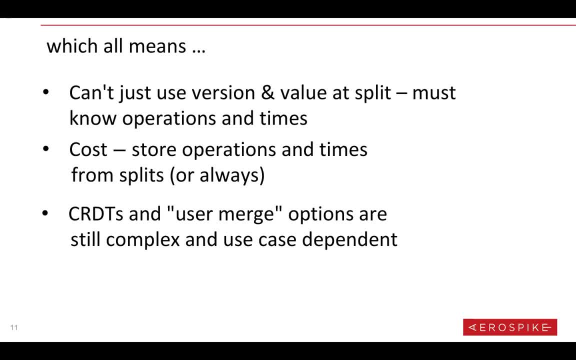 or a use case where it can recover things in a limited fashion. only for that use case, Some CRDTs will even actually lose data on the merge, And you know that that doesn't even give you the so-called eventual consistency. 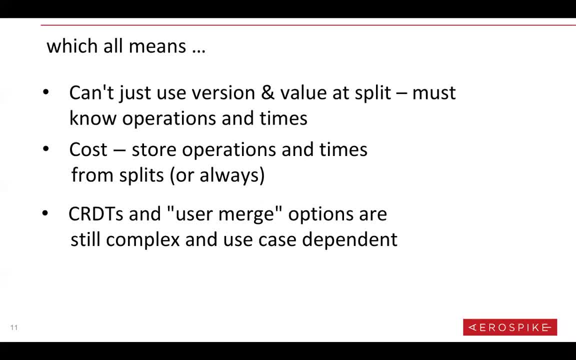 It's just a controlled or stated way of of how you want to lose your information, how you want to lose your rights And in general they're also very complex. you know complex things And you know for a high throughput. 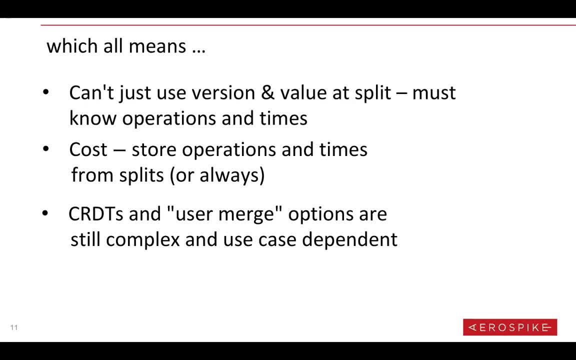 high, low latency, high a large scale database like Aerospike, you know, something like this would be a big challenge. So, in general, eventual consistency for for a lot of databases is going to be a pretty extravagant cost. So when we were faced with a choice, 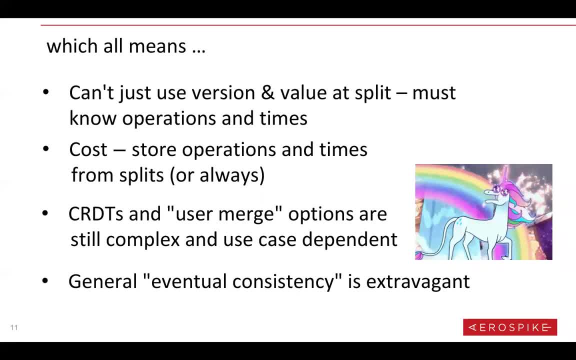 we, we actually chose to to do strong consistency first, or so far it's really the only one we have, because strong consistency, unlike eventual consistency, is actually use, very use case independent. It doesn't really matter what your use case is. 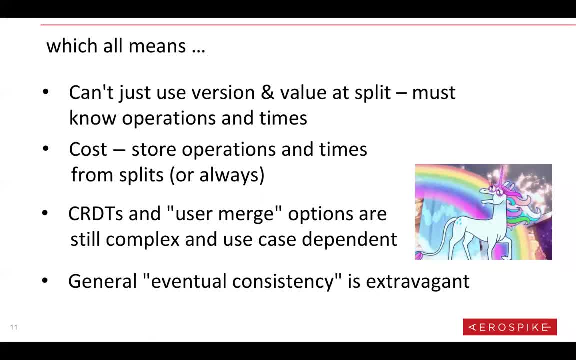 You're going to get your guarantee. It has its own challenges, of course, which we will now get into, But but I just wanted to clarify that eventual consistency is absolutely not strong consistency. They're very different things and they take very different strategies and implementation. 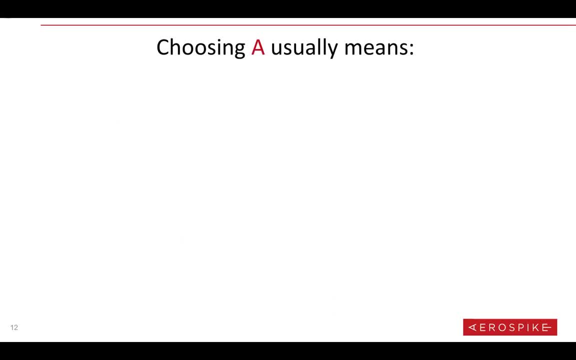 Okay. So again to recap, if you're choosing a high availability database, it'll generally mean that when we resolve your conflicts in these split brain scenarios, what will happen is you're going to lose a right, You're going to lose something. 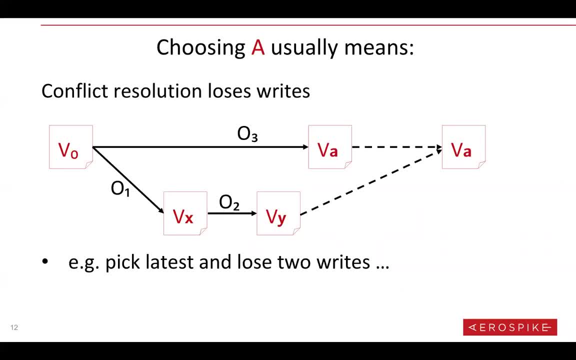 So in Aerospike, for example, we we we allow you a choice of two very simple schemes of merging records back from splits. One is that you'll just pick the latest. The other is that you'll pick the one with the most history. 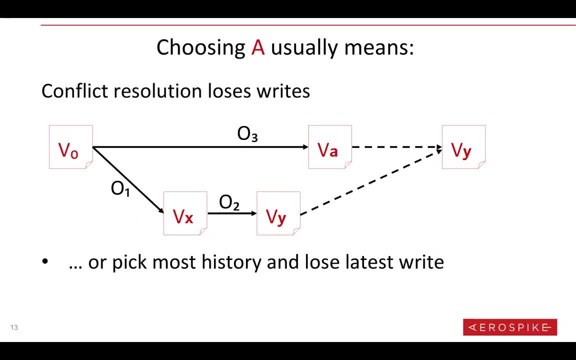 which, by the way, a lot of ad tech, a lot, Well, a lot of our customers in general choose this option because usually, if you're merging two things back- and one of them is the entire history of the record that was there And the other one is just- 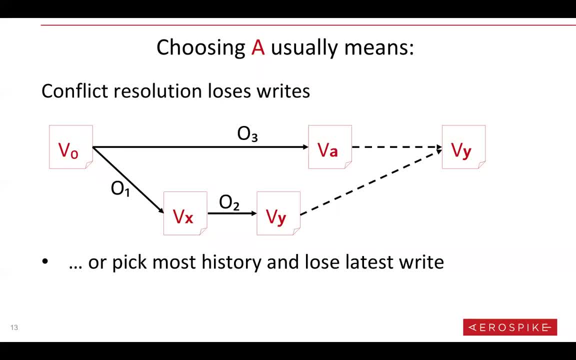 this spurious new little stub of a record that was created in some branch And it happened to be later. You don't want to wipe out the bulk of your information, So they would rather lose the, the later single right or very few rights than the. 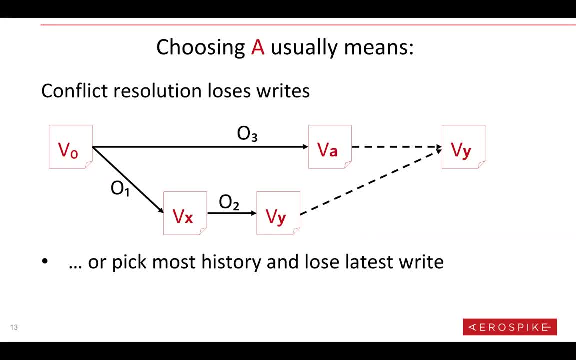 than the slightly earlier but containing much more information record. By the way, notice also to go back to this slide where we, where we pick the latest. Sorry, I guess I have to go to back, Yeah, where we pick the latest. 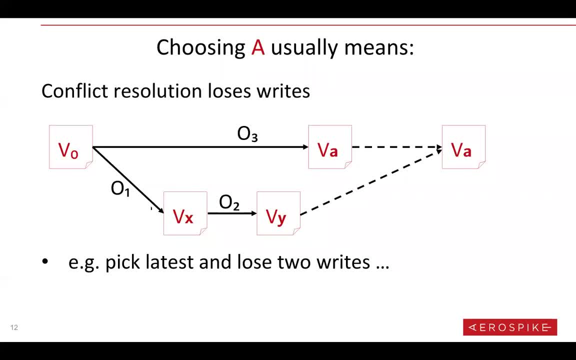 If my usage model happens to be that every operation simply replaces the record and doesn't depend on the previous value, Well, Hey, this scheme gives you eventual consistency, because this is exactly what you would have seen if, if the split didn't happen on these, things happened in this sequence. 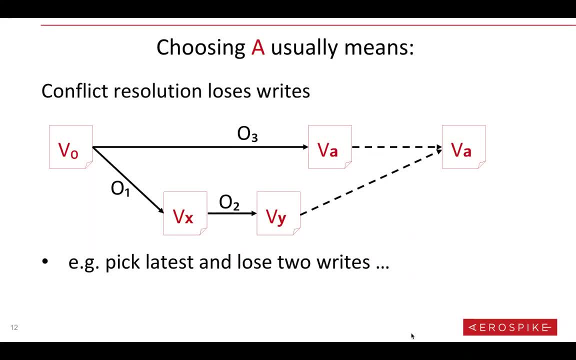 So I'm just saying that to point out that the ultimate use case Dependence of eventual consistency. So yeah, we, we do eventual consistency: consistency for the use case where, where you just replace records and don't care about the previous value. 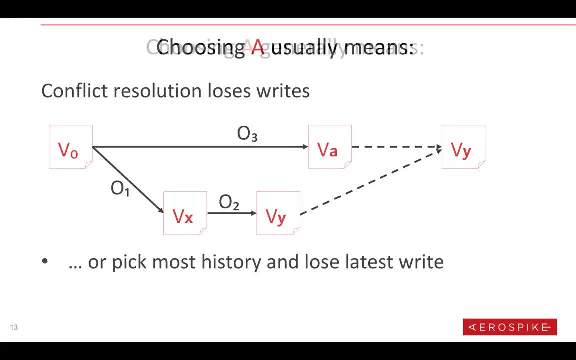 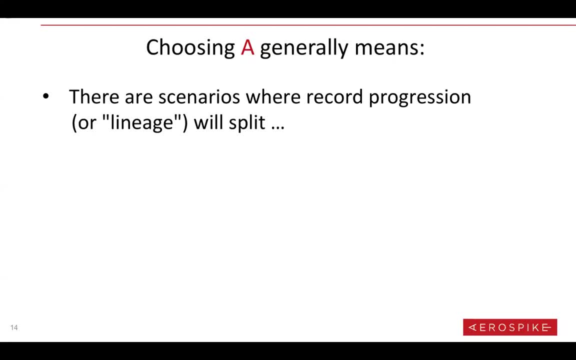 which, admittedly, is not that common a use case. Okay, So if you choose a, what it means is that they're going to be scenarios eventually, someday, where your record progression will split and it'll be observable. This split, In other words, you, you're going to be allowed to do rights and reads on the split values. 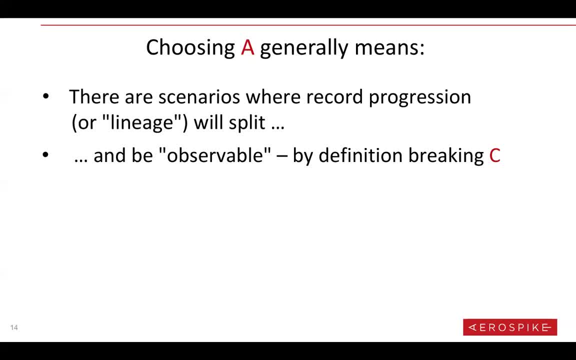 And by definition you've broken my definition of strong consistency, that that single linear sequence, and at the end you're going to end up doing conflict resolution of your split lineages. and either it's going to be very complicated and require storing lots of history to get back the best version that you possibly could. 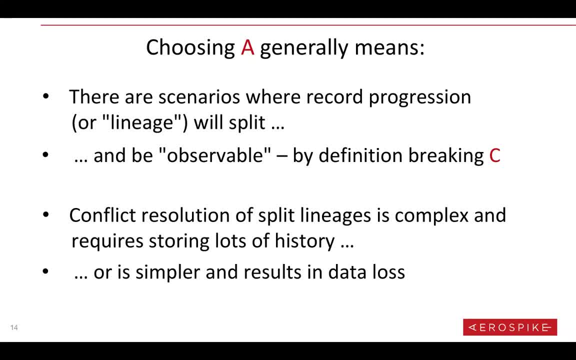 Or it's going to be something much simpler and cheaper and that will result in data loss, or both. So there's your high availability And again, we, Aero spike, had only this mode for years and we did quite well for a lot of use cases. 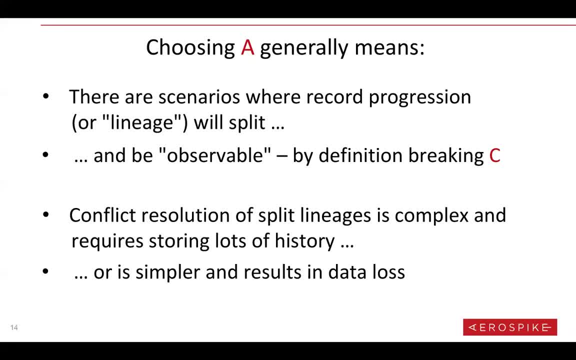 This is what people want. They don't really care if they occasionally lose a little bit of data. They invest their efforts instead and in just trying to make sure That the scenarios in which this happens are minimized. get the best network You can, manage the cluster the best you can and and hope that Aero spike writes good code so that their nodes don't crash all the time. 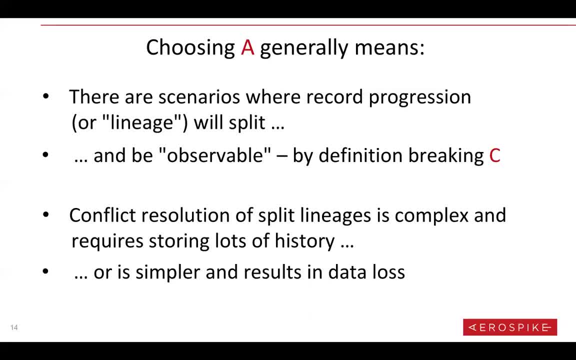 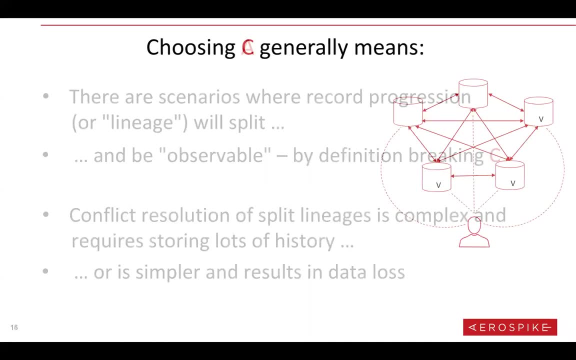 And it, for many customers, has worked fine. They can run for months or or years and they they don't really get any of these scenarios and they don't lose any data But again someday when the scenario happens for some use cases. it's just not going to be acceptable. 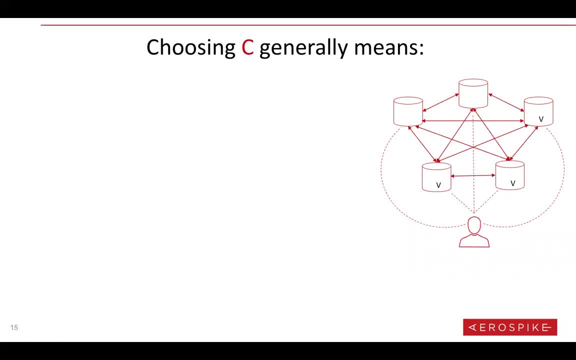 Okay, choosing strong consistency. What does that mean? The strategy in general is to disallow operations that would cause record version splits. So, for example, here in the picture, as you see it, if, if I can only see a piece of the cluster, 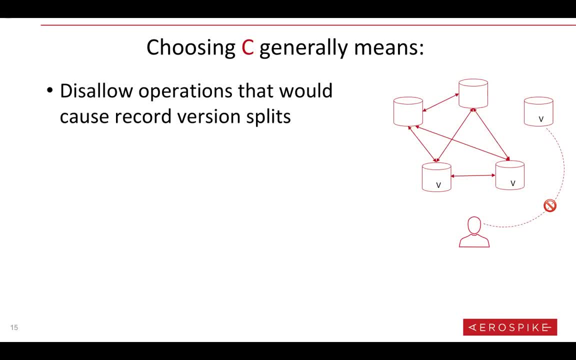 and I know that this is going to cause a version split. I'm just going to not allow you to do the operation. The other thing is you have to disallow observations of of dirty versions that somehow do get there, when they would cause a split. 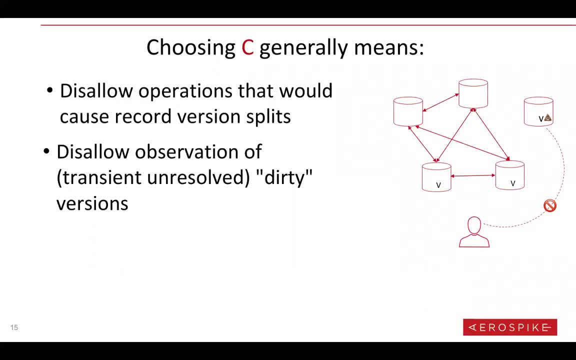 And just a word on that: in general It's pretty hard to avoid getting dirty versions- What we call a dirty version- In any system, because in general you can commit a right on a node at a time when you know everything is fine. 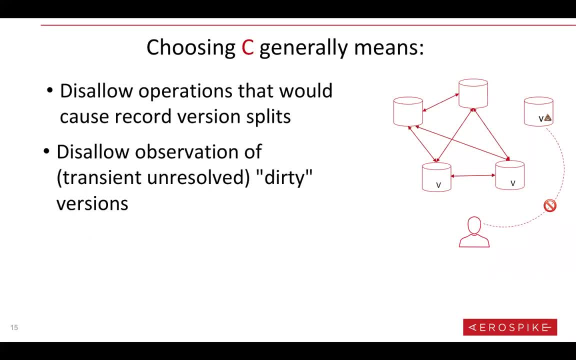 But before, before you can finish the whole transaction, all the replicas of the on the nodes that they, that they need to go on, then something goes wrong and you actually are end up, at least temporarily, with this version which is, which is dirty. So the corollary of disallowing operations that would cause record version splits is if something does somehow get in there. 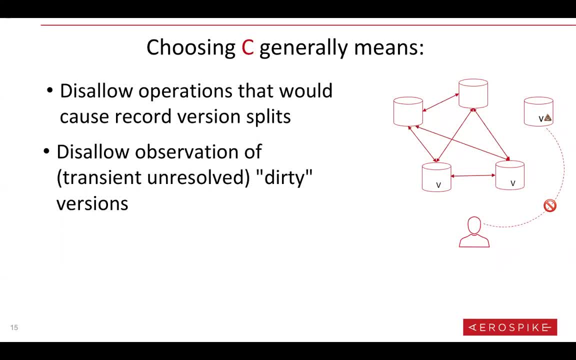 That would cause that you have to disallow observation of those versions. So you have to know when they're. when they're dirty and pretty much not not let them participate in the in the database activities. So that is pretty clear that if we're going to do this, 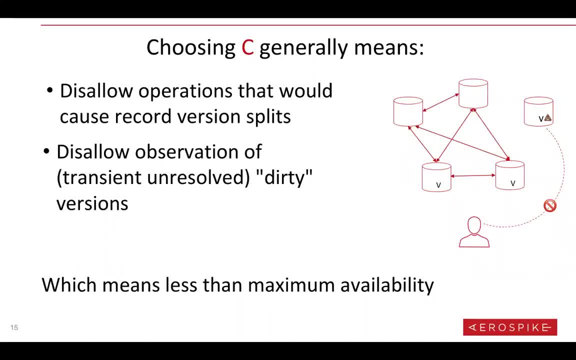 we're going to be disallowing operations on nodes, which you can see from an application. by definition, I'm violating my maximum availability premise. So there is where strong consistency is going to, to give up availability because we are literally going to stop you from doing transactions that will that will cause splits. 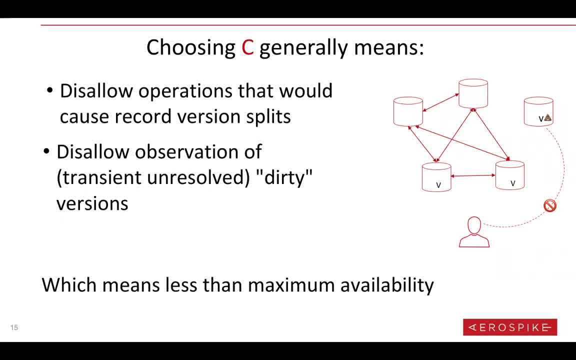 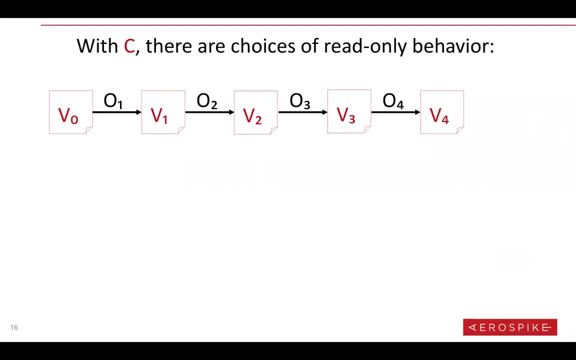 Even when we can see a node that we would otherwise, in a high availability scenario, done a transaction on Okay? I said at the beginning, when we gave the definition of strong consistency, that there were choices of read-only behavior. So what do I mean by that? 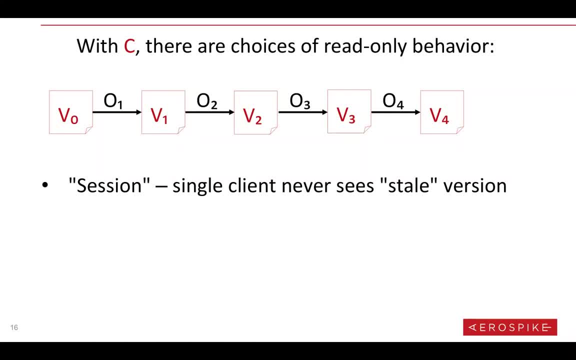 We've established that for sure. We're going to have a single linear progression of the record version, And our first mode that I'm going to talk about, which we call session consistency for reads means that a given client, a given view of the cluster, will never see a stale version, meaning that you know. 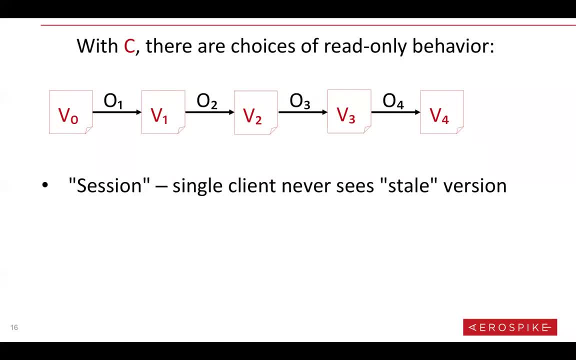 if it did a right. if it did it right, Oh four, and created version v4.. It can't do a read. that would then see version v3.. Now there is a stronger version of of read Sequencing, which we'll call linearized reads. 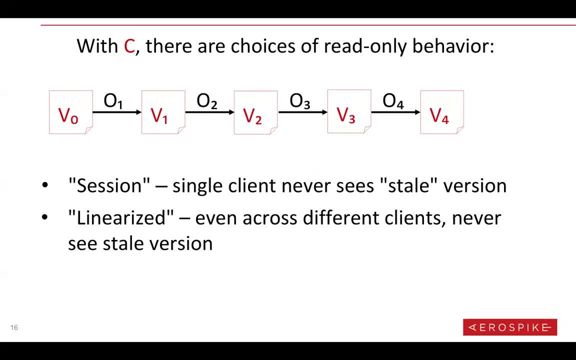 which means that even across different clients, we can never see a stale version, meaning that even if client a wrote operation for and created version for, if client B reads that record after that, it has to see version for it can't see version three in session consistency. 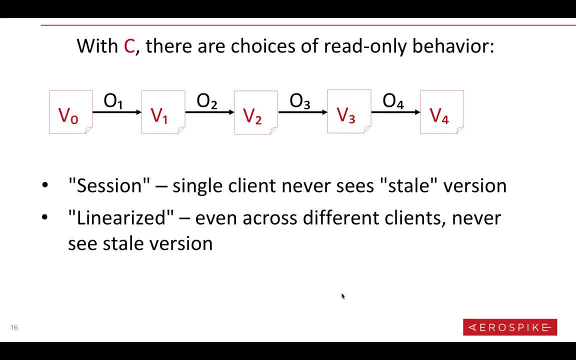 It might be possible for client a to write version four, but client B then goes and reads and finds version three because it's it's a map, hasn't caught up or whatever the implementation detail is. So, while the single client will see a linear sequence and never go back, if you actually had a way to for a and B to compare notes. 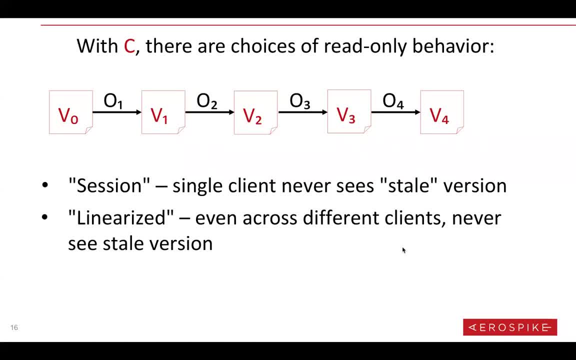 you would find that that one managed to do a right and the other one, after after that right, didn't see the right. now a lot of people Ask. Well, before I get to the difference between those, there's a third version which we in aerospace support. 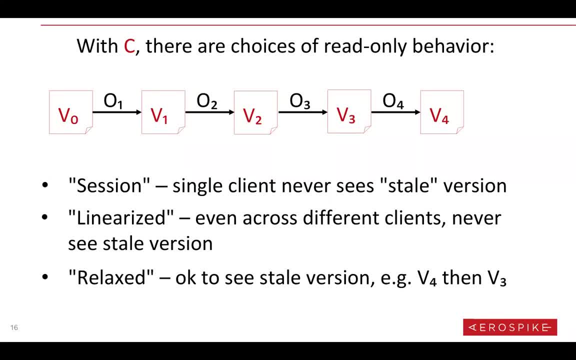 which is what we call relaxed, where it's perfectly fine to see still versions, even in a single client. The main care is that rights are never lost. They don't really mind if occasionally you see a stale version in the in the single history, But yeah. 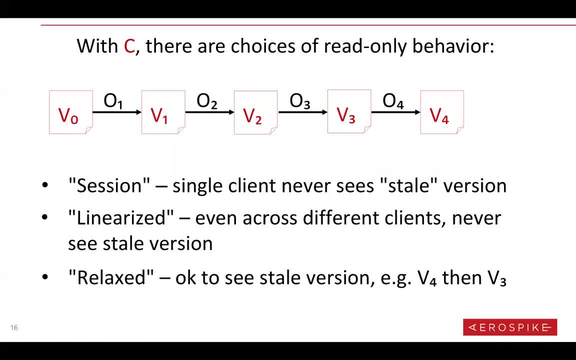 one of the most Common questions We get asked as well. Should we use? should we use the linearized mode, which, as it turns out, has a pretty high performance cost as compared to session mode, and the best answer I can give is if your clients actually do have a way to compare notes with each other. 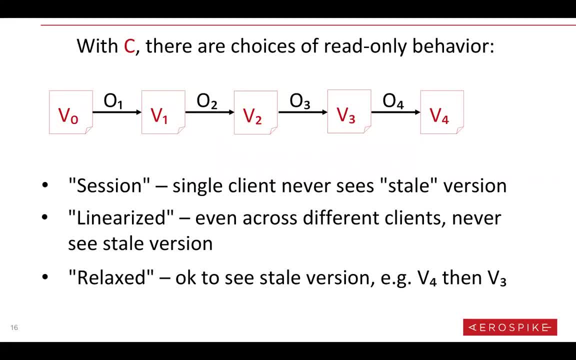 Then maybe you want to think about it. if they have a way to compare outside of aero spike, but if there is no source of or no way for them to to compare notes or no source of truth outside of aero spike to verify that they were in sequence, 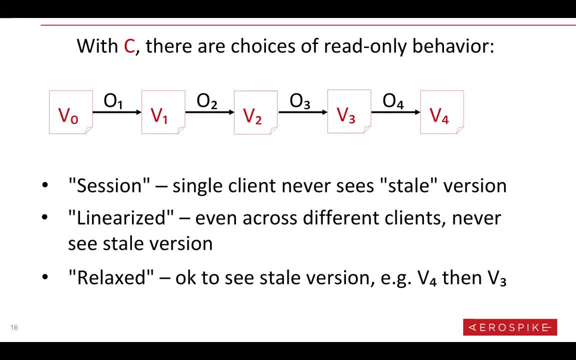 then pretty much that means that then you don't really need the linearized mode, because if you can't know about what the other clients saw, then it really only matters What what you, what one client sees, and then you can go with session consistency. 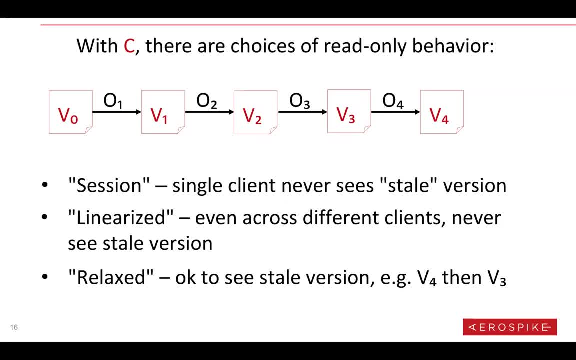 which, by the way, is does seem to be the mode of choice for many of our customers. Okay, so yeah again, that none of this changes what we said earlier about not losing rights. We still have this single history If you're doing a read as part of a right. 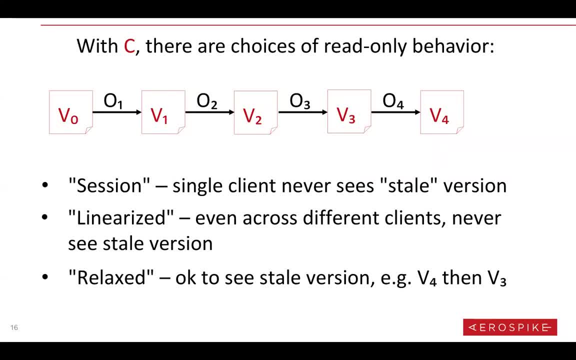 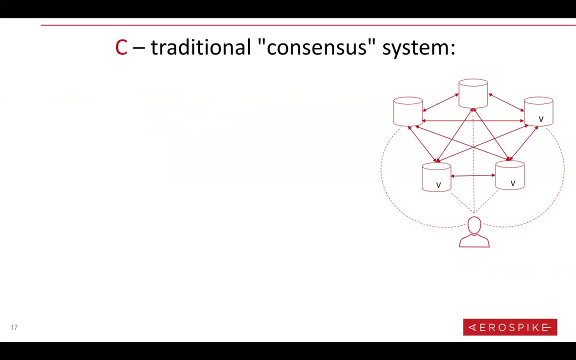 you know that obviously has to be in success in the succession of the rights. but these are read only ordering concerns and that's what these modes are all about. there There are purists, by the way, who will tell you that if you're not doing linear, linearized reads. 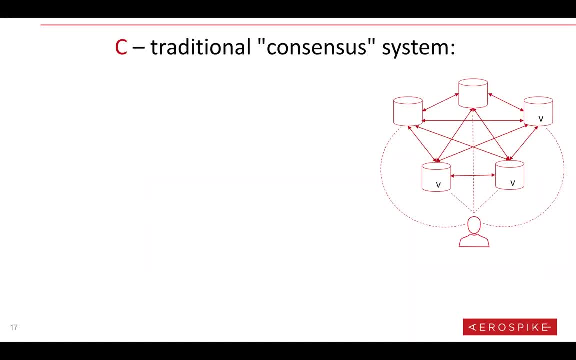 you're not really doing strong consistency and we could argue about that, But occasionally you will look that up and you'll see that that's included in definition of strong consistency. But for me it's not. to me It's about losing rights. 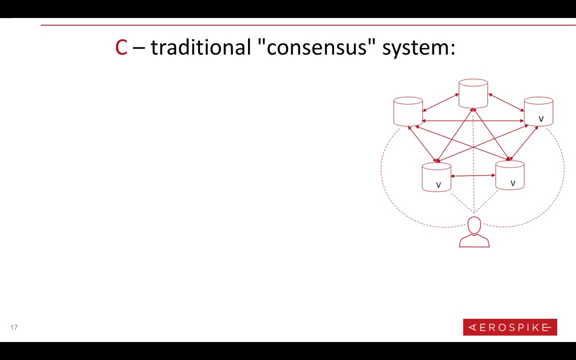 Okay, A traditional consensus system. So I'll talk a little bit here about traditional strong consistency implementation versus ours, again mainly to highlight that you can do this different ways and get the same guarantee. So to quickly run through it: a traditional consensus system. 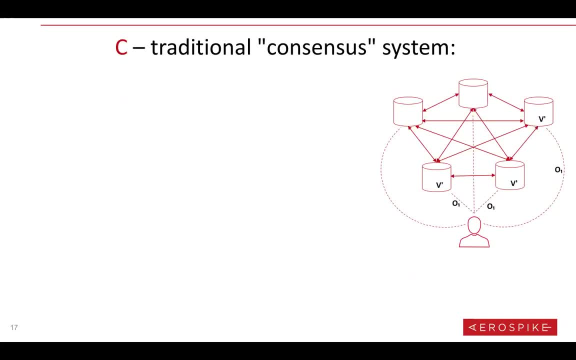 you'll have stationary versions, What I call stationary versions of a given record in a cluster. In other words, you'll always have certain nodes designated to be the nodes on which a given record sits, And when you do an operation, the operation is done in parallel, generally, to all those records. 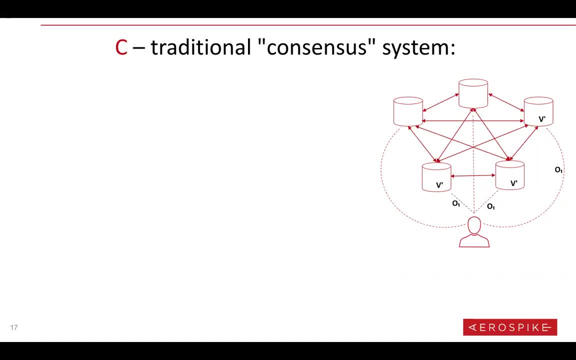 So your operation there went straight from your client to these nodes. by some means it doesn't have to go straight from the client, which, as you'll see in some implementations can provide an advantage, But the idea is that you write all three independently. 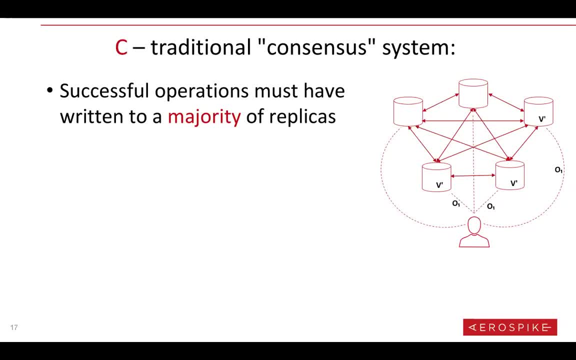 and you probably have a two-stage system to verify that they all got written, And a successful operation must have written to a majority of the replicas, which actually has a corollary meaning that for you to have a hundred percent availability with n nodes missing, 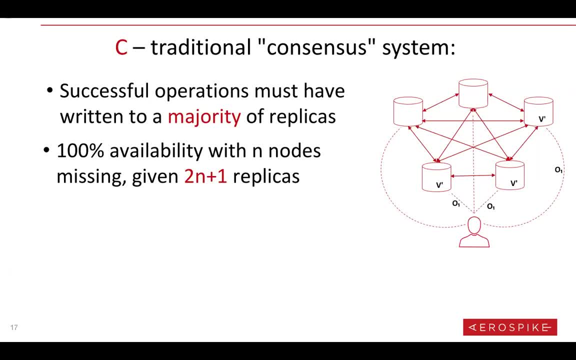 you need to have two n plus one replicas. So here for me to run with a node down with one of those three versions missing. obviously, to get a majority I need two of three, So I'm going to need at least three replicas to be able to run with one. 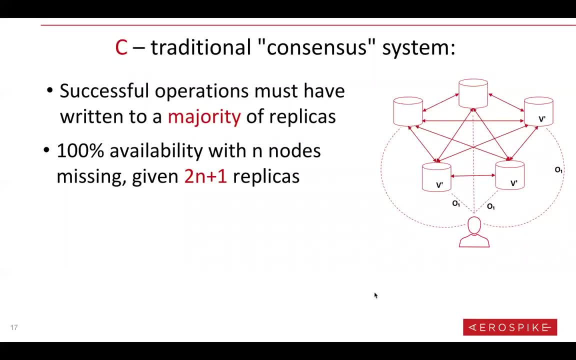 one node down. If I had two replicas and one node was down, I wouldn't have a majority anymore. So we have that constraint. It also means another corollary is that you need then at least three replicas to be able to do rolling upgrades with a hundred percent availability. 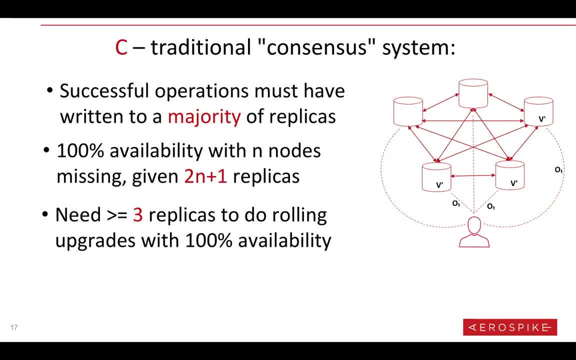 because the best you can do is take one node down at a time. That's the fewest nodes that you can take out at a time, And so, if you want to keep your availability, you're going to need a minimum replication factor of three. 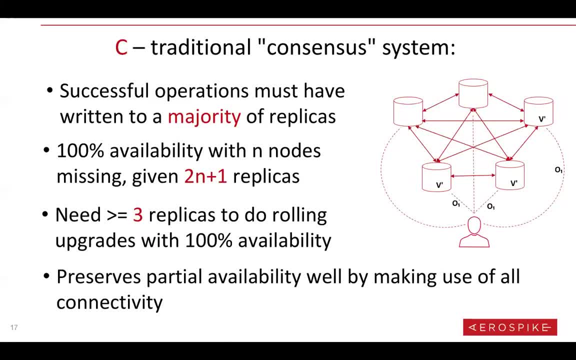 Now, one good thing about most consensus systems is they preserve partial availability really well by making use of all connectivity, Good implementations of this- you can chop out all of those, a lot of those connections, and as long as there is any path from your client that can get to the three. 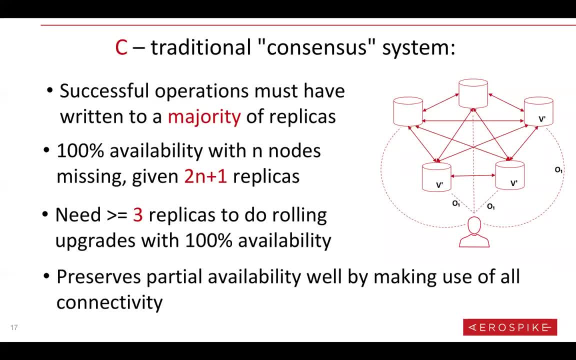 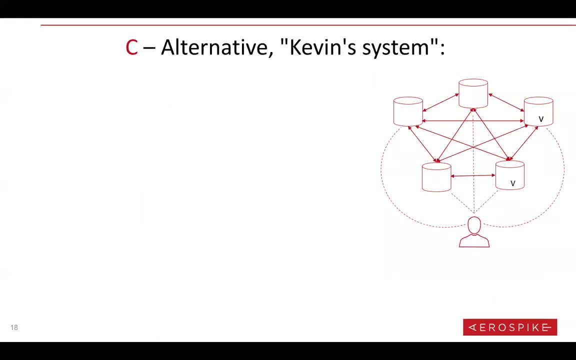 or the however many replicas that sit on different nodes. as long as there's any path to get there, then you can succeed. So you can actually withstand a lot of of of connectivity breakages. Okay, so now I'll briefly describe the way we do it in Aerospike. 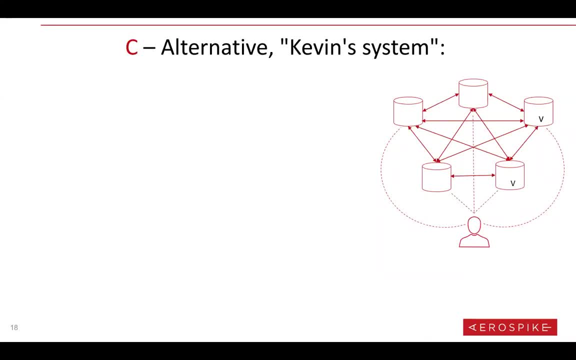 just to highlight some differences. And yeah, here Kevin's system means Aerospike, because in the original talk I was not allowed to mention the the name Aerospike- and Kevin's one of our engineers who played a major role in designing this system. 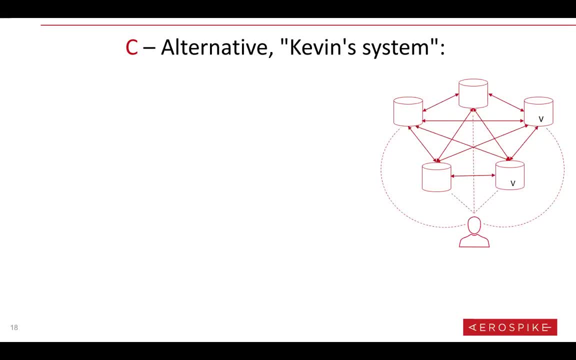 But in Aerospike system we'll only keep two replicas, as compared to three in the other case, And the way that our operations go there, it's master centric. The operation will go first to the master and then it will be replicated to. 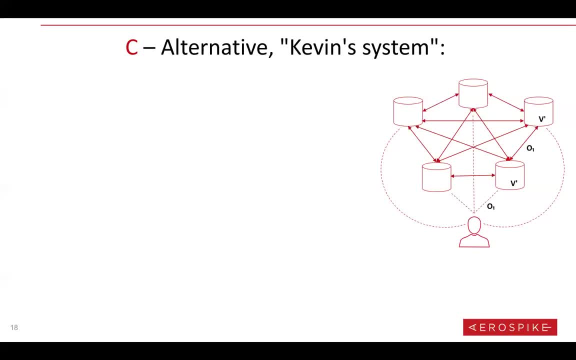 to whatever you want to call it. We call them proles, slaves, replicas. Then it will be replicated to the other node, So they're not independent. It definitely goes in this order And just like in. just like in the traditional consensus systems. 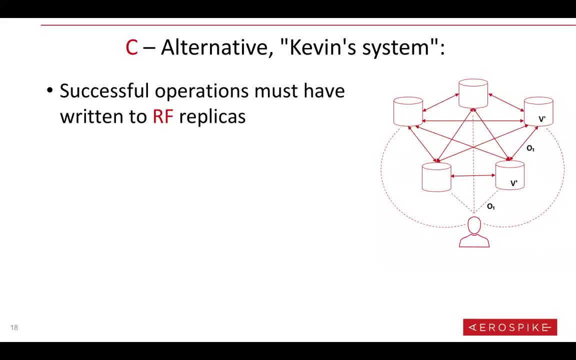 we do have a requirement that a successful operation must have written to replication factor replicas. But in this case- notice here- all we're saying is it's just that many replicas, It doesn't actually matter what nodes they're on. And in our case, 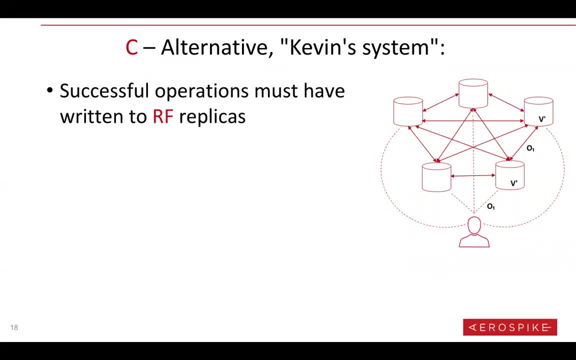 we don't necessarily always have both the replicas on the same two nodes. If the cluster changes, other nodes will fill in to, to stand in as replicas or masters, and and then we'll end up being able to complete- complete a transaction as long as we can get to. to enough of the nodes. So what that means for us is that we can have a hundred percent availability. One corollary is with only end nodes missing If we have N plus one replicas. So that means, for example, that we only need two replicas to be able to do a rolling upgrade with a hundred percent availability. 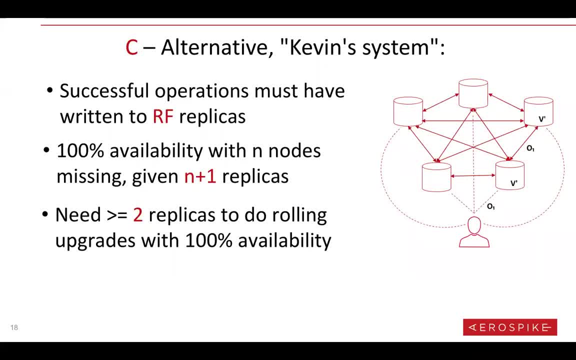 So that turns out to be quite a big advantage, obviously for for cost, If you really only need to carry two replicas instead of three to be able to keep your a hundred percent availability. And on the downside, what we find is, while we maintain a hundred percent availability, 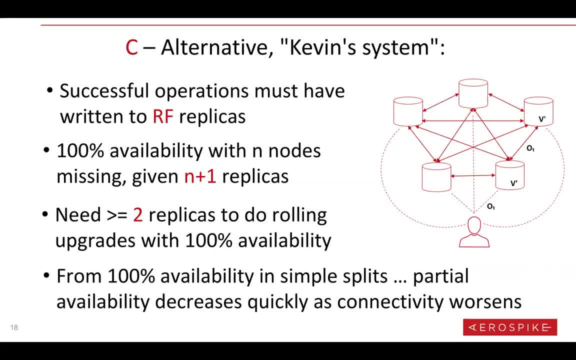 perfectly well in these cases, with fewer replicas and in very simple splits, our partial availability as compared to a traditional system will decrease quicker as connectivity worsens. So we can actually get scenarios where you know, if you chop out enough connections we'll have. 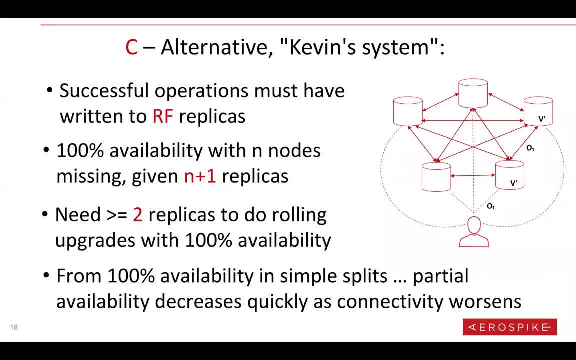 we'll actually go all the way to zero availability, where a traditional consensus system might, might retain quite a bit. So there there are some trade-offs, but we think they're good. Okay, The trade-offs again. just to summarize is that: 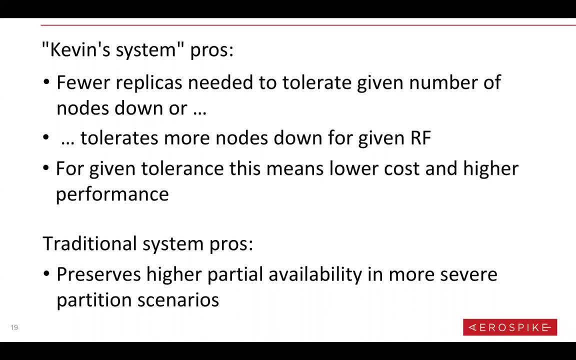 in aero spike. we need fewer replicas to tolerate a given number of nodes down and maintaining a hundred percent availability, or we can the opposite: we can tolerate more nodes down for a given replication factor, So for I could have replication factor three. 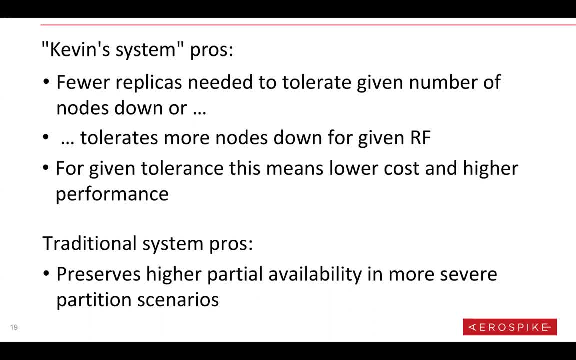 I can actually take two nodes down at a time and maintain a hundred percent availability, Whereas it would be one for a traditional consensus system. So for a given tolerance, whichever way you want to do it, it just means that you're going to end up with lower costs because you're carrying fewer replicas and higher performance again. 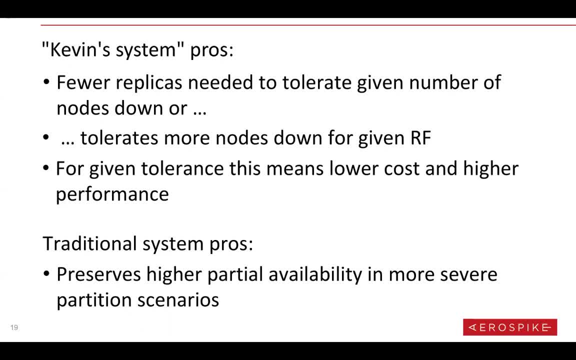 because you're carrying fewer replicas. So there is just less work to do to do a right. There's just less going on in the system. Traditional system advantages, as we said twice before, is that they're generally much better at preserving partial availability and more severe cluster partitioning scenarios. 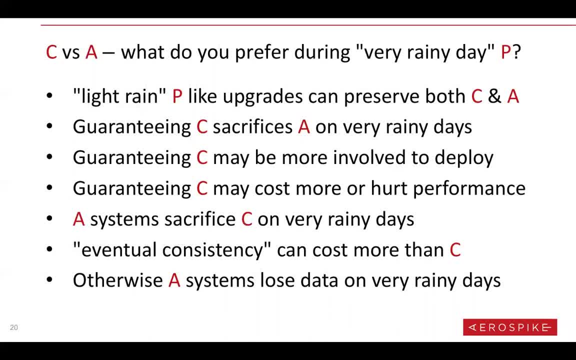 Traditional system advantages is that they're generally much better at preserving partial availability and more severe cluster partitioning scenarios. Okay, getting near the end, now the final recap. the choice of C versus A really is about. what do you prefer during a very rainy day? 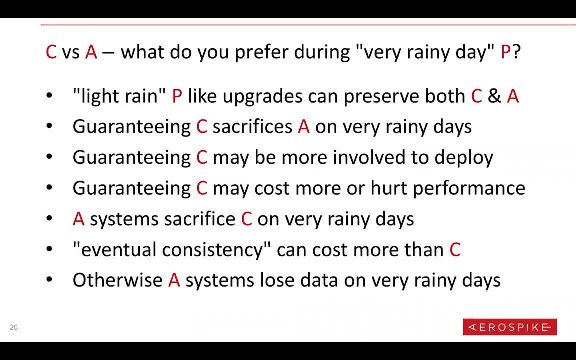 cluster partitioning scenario. And remember it has to be very rainy. If it's light rain, just meaning like I take nodes down on purpose to do an upgrade, or one node goes down by accident, Most systems will give you both for free. 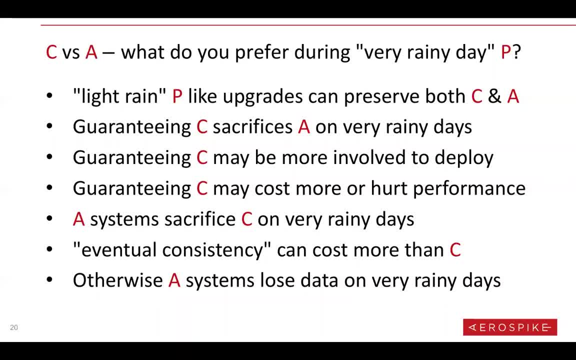 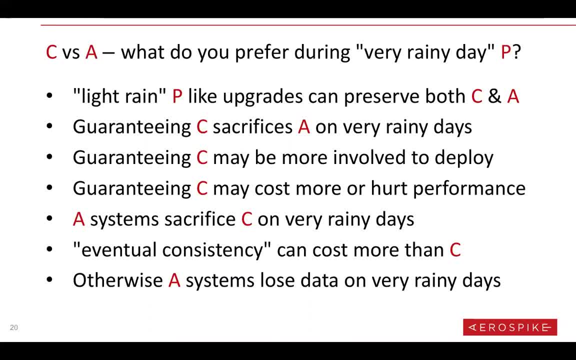 So guaranteeing C, if that's the choice you make, you're going to sacrifice A on really rainy days. It may be more involved to deploy, For example, our strong consistency system. you have to manage a roster. The cluster has to actually know what nodes are supposed to be in it. 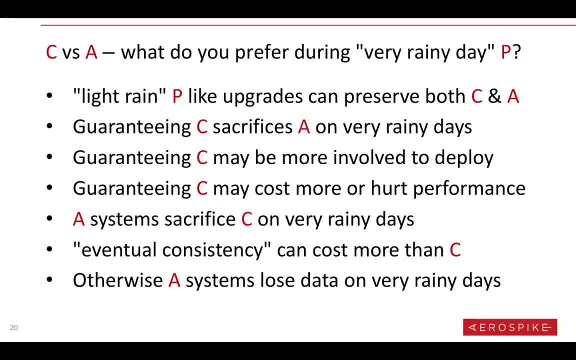 where our high level nodes are supposed to be in it, where our high level nodes are supposed to be in it, where our high availability mode. you know, everything is very free about that. The cluster just develops in terms of what nodes can see what nodes, and you don't have to specify anything. 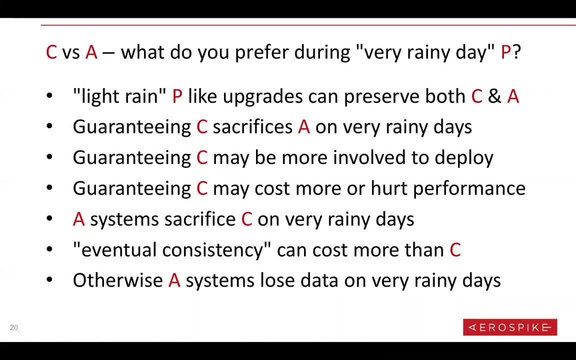 So there is a little bit more operational play involved. Sometimes it can cost more or hurt performance. In an aerospike system it has almost no cost. In fact replication factor 2, it pretty much does have no cost. But in a lot of other systems it is going to cost you more, if for no other reason, by making you carry more replicas and do more work per write, But it doesn't have to. I mean, we do a pretty good job of that- And high availability systems. 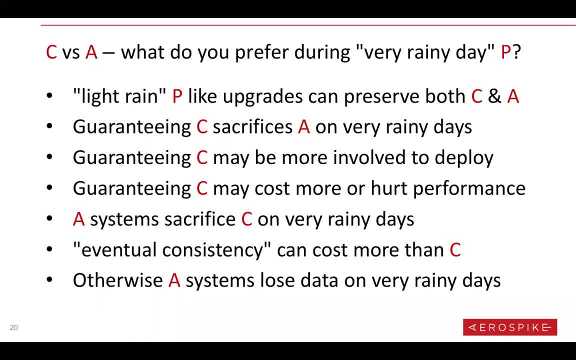 which sacrifice strong consistency on very rainy days. Again, notes to remember: eventual consistency is a complicated thing. It it can actually cost you more than strong consistency in terms of complexity or performance, But otherwise you know, if you keep it simple. 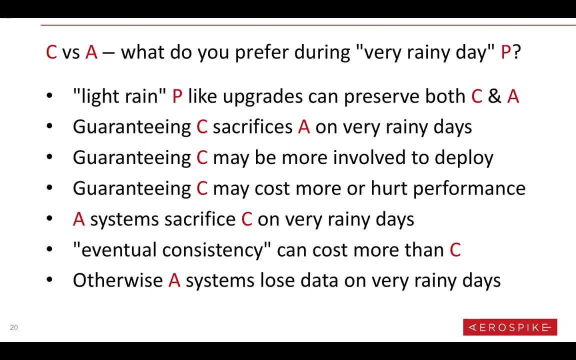 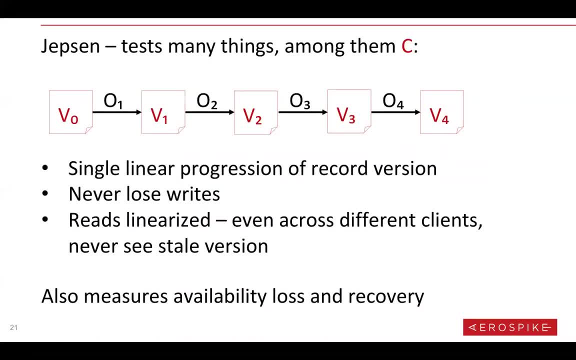 then your, your high availability system is going to lose data on on your very rainy days. So that's the choice you're making, And that's pretty much it. This is our optional slide. If you guys want to hear about this, I'll. 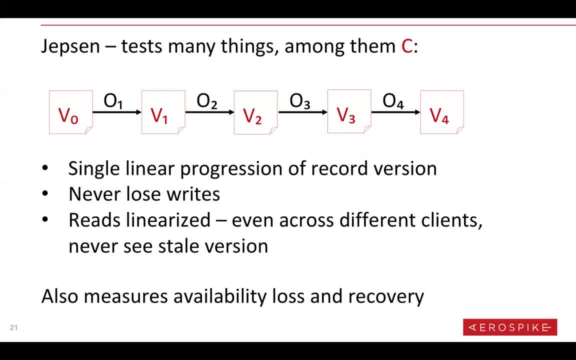 you, we can. we can address it in the question session, But in for the talk in Israel. people wanted to hear about this. There are these tests done by Kyle Kingsbury, where who's an independent contractor that goes around and tries to to ensure or debunk your claims about whether your database is strongly consistent. 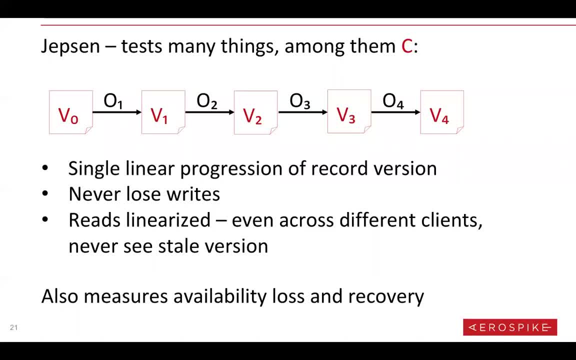 He came to us and tested everything we claimed And we passed the test, which is not a trivial thing to do. So if you're really considering using strong consistency, you should probably go and and read that and at least be happy in the fact that a third party is telling you that- that our claims seem to be true. 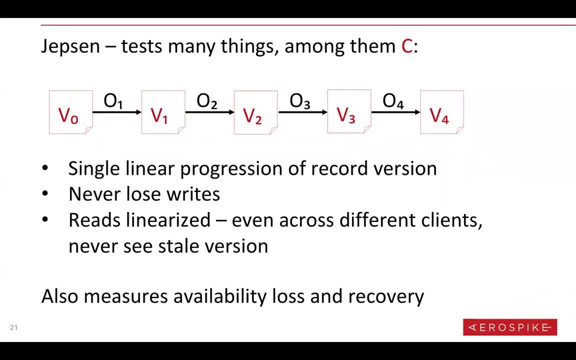 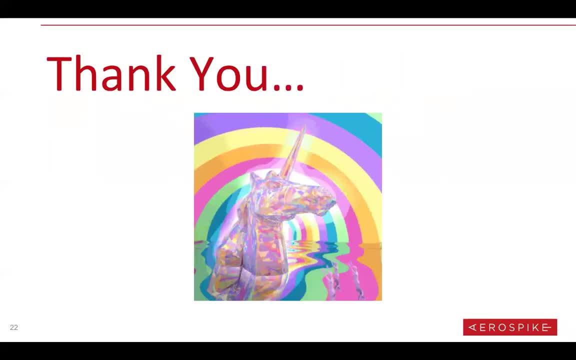 And that this isn't just salesmanship. But if anybody has any questions and details about that, you know, feel free, We can talk about it afterwards And that's it. Thank you very much. Now I'm going to see how long I took. 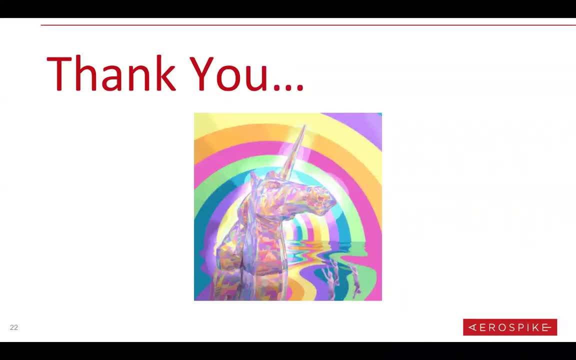 Thank you very much And the for the talk. Okay, There are no questions in the chat, but I'm changing the settings so that anybody who would like to ask a question is now able to unmute themselves and present a question. So please go ahead. 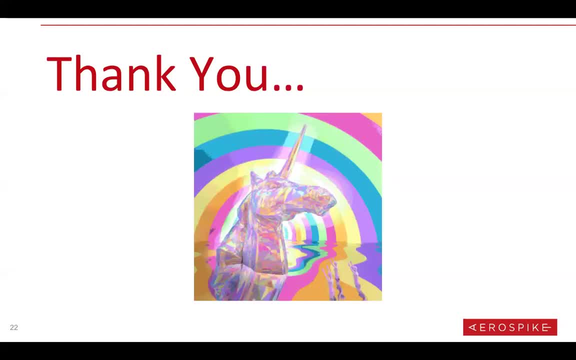 If you want Andy to create the more flesh, maybe you can bring back that slide. Is anything happening, Natalie? Nothing is happening, So maybe you can bring back the slide that you just mentioned and discuss about that a little more. Well, we can talk about. 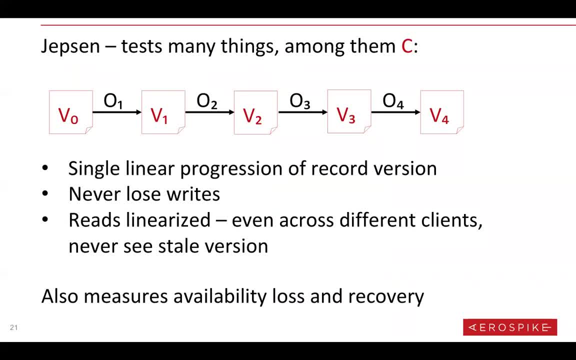 Any slide, The one that you mentioned. You're thinking to add more details depending on how the questions go, So maybe we can. I mean, if people want to ask specifically about what the Jepson test is and and what it does and our experience with it. 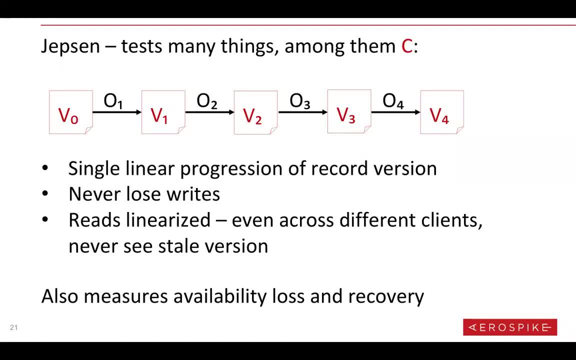 I'm happy to to talk about it, but I'm happy to talk about anything else too. All right, First question actually came in in the chats: What does strong eventual consistency mean? It's a term I heard related to CRDT. Yeah, 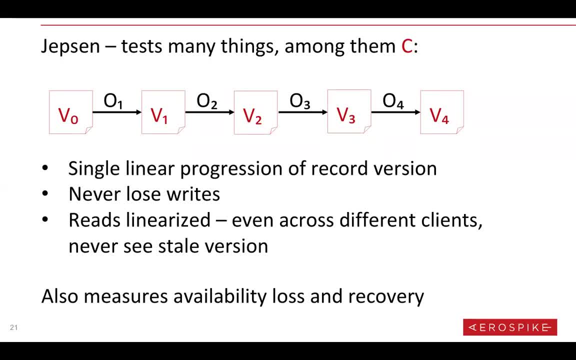 so I I don't really understand why they, why they put the term strong on eventual consistency. What I described as eventual consistency, I think, is what they mean. Actually, I think they may mean even they. They may mean even less, because if it's who, I think it is. 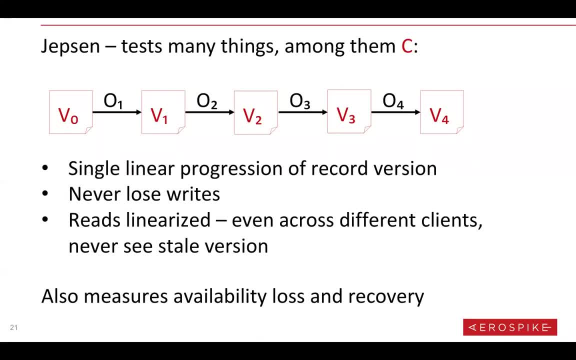 it is an eventual consistency for particular use cases, as done by a CRDT, but I believe these CRDTs also will actually force you to make a choice as to how you lose data in certain merges. So to me that doesn't even qualify as eventual consistency. 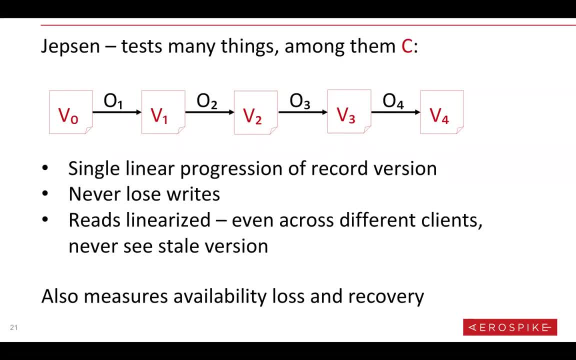 but I don't know what, what the intent is. to add the word strong to eventual consistency. You're either eventually consistent or you're strongly consistent, And I don't. I don't know that there is an official definition for a strong eventual consistency. The strongest it can be is that is, you know, to go back to. I can find the slide. 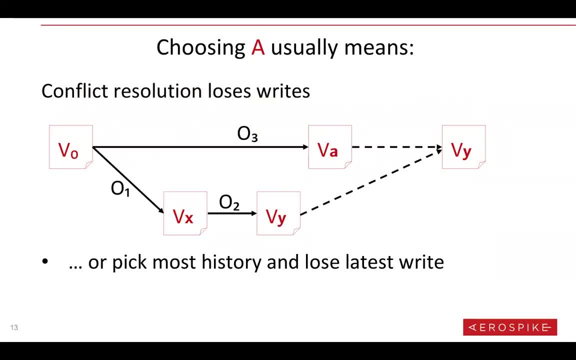 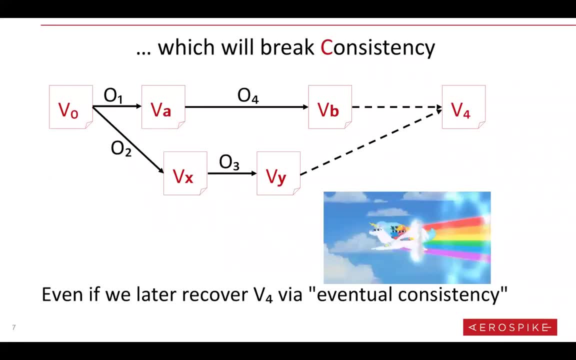 The strongest know it's further back. So, yes, here the strongest it can be is that, in general, anything that happens here, When the merge happens on the smoke clears and the cluster reforms itself, You end up with exactly the version that you would have had if none of this cluster split situation happens. 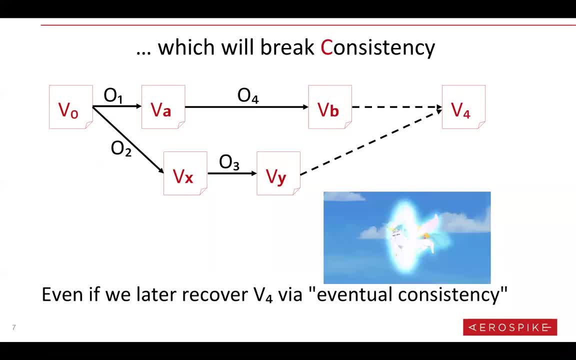 And that is that's as good as you can do in terms of eventual consistency. So there's nothing stronger than that, and achieving that in general is unbelievably hard If you have CRDTs, almost certainly. the CRDT is specifying a certain use case or usage model. 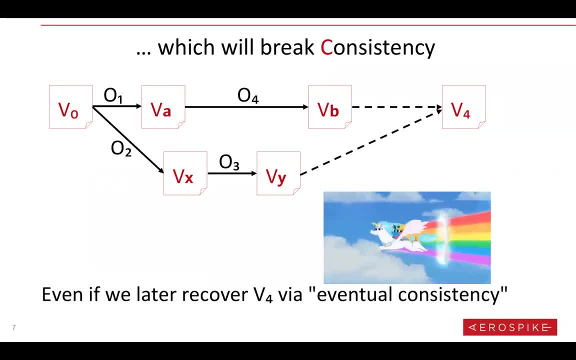 Like it might be saying if you're doing in numerical increments or whatever else that it covers, And in those cases it might be good enough to actually do this, which is what I would think I would call strong eventual consistency- If I was going to put the word strong- or it might actually cause you to make merge choices where you do lose rights. 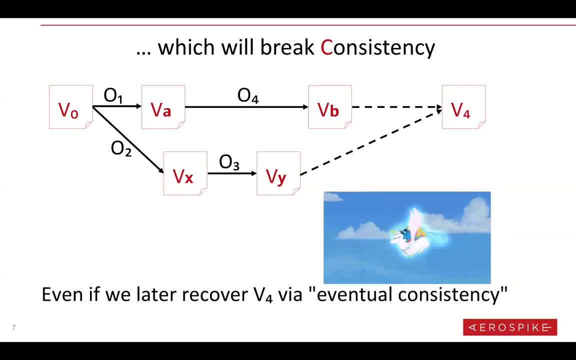 In which case I don't even understand why you're calling it eventual consistency. It should just be, you know, eventual conflict resolution, because if you've lost anything you're not really consistent. So yeah, I don't. the answer is: I'm not really sure what they mean by that. 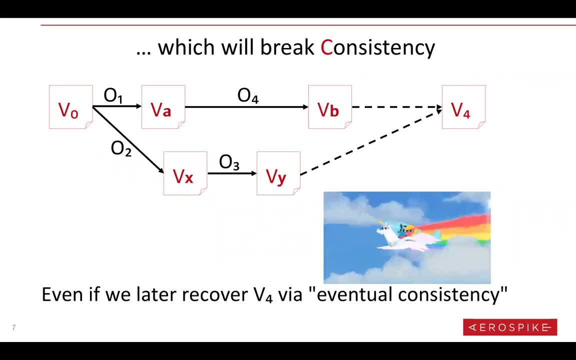 but I'm guessing there's really no distinction between that And what I described in general. Thank you, Are there more questions? You're welcome to ask about the talk. You're welcome to ask about your spike. Yes, anything goes. Well, then the sketch note is actually being already shared and ready. 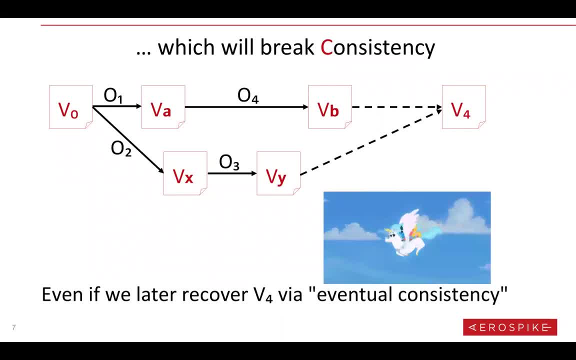 So that's great. Thank you for showing it, Miriam, And looks like we're coming to the end of our event, So if you want to ask questions afterwards, you're always welcome to join our forum. or read it easy to Google and we will be there to answer questions.